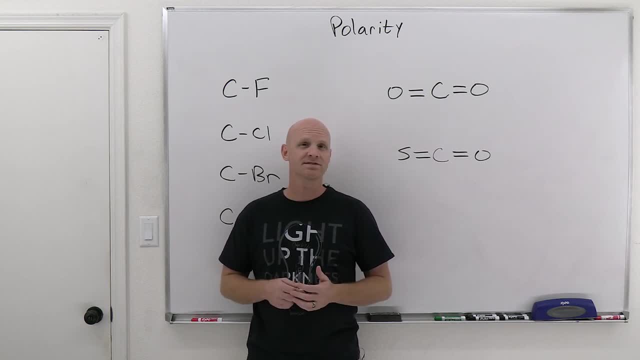 I'm covering an entire year of general chemistry, releasing several lessons a week. so if you want to be notified every time I post a new one, subscribe to the channel, click the bell notification. All right, so quick review. You might recall that fluorine was the most electronegative element on the periodic table. 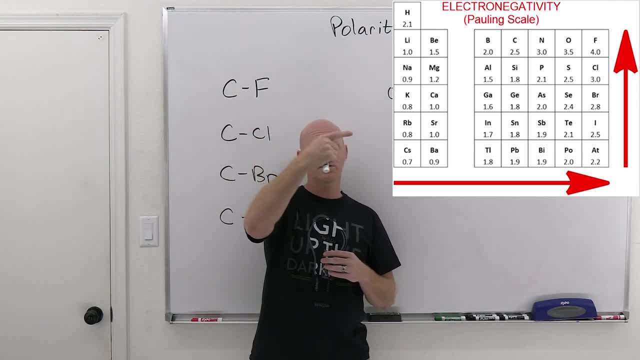 and the closer you get to fluorine, either going up a group or across a period from left to right, the more electronegative the element. And you're supposed to remember that fluorine's number one and that oxygen's number two. 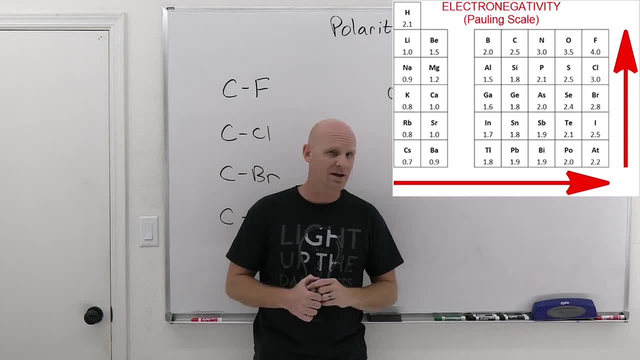 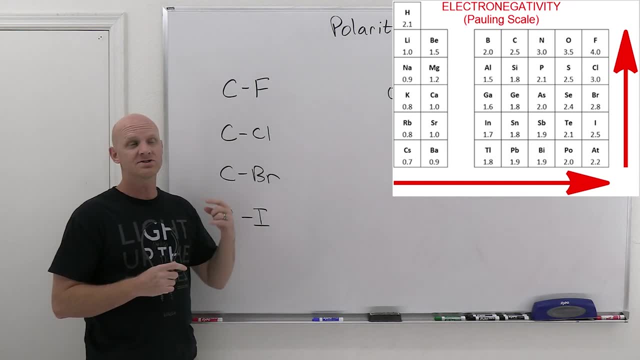 and after that suffice to say: the closer you get to fluorine on the periodic table, the more electronegative an atom is. Now, in identifying polar bonds, we learned a couple of rules. We learned that if you've got two identical atoms bonded together, 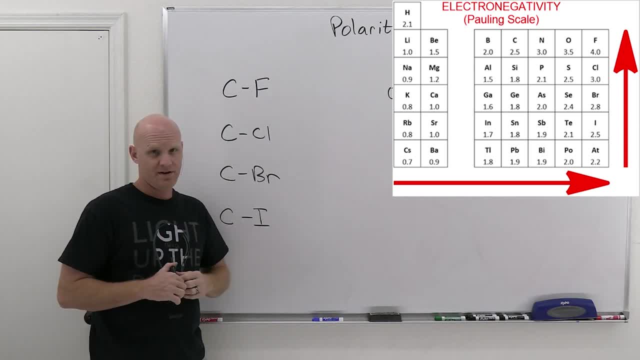 that's typically going to be nonpolar, or carbon and hydrogen. And we also learned that if typically the difference in electronegativity was less than 0.5, we'd call it a nonpolar bond. but unless you're given the Pauling scale of electronegativity, 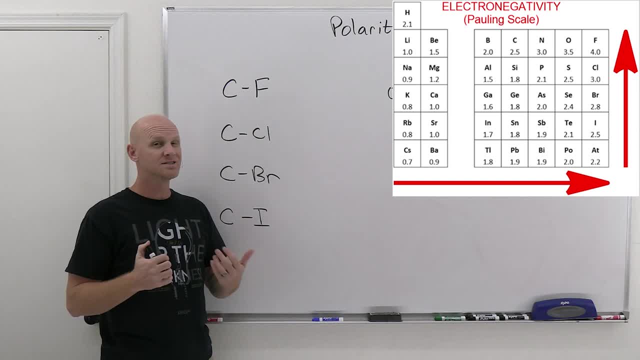 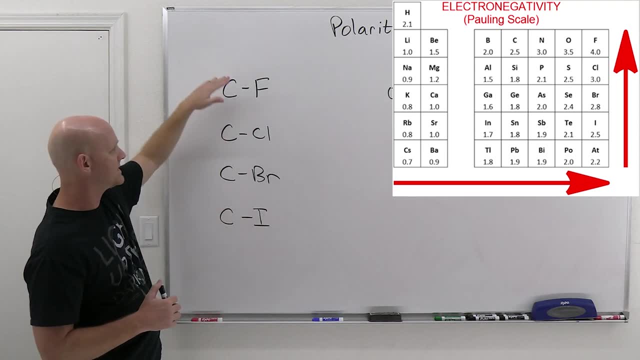 electronegativities. you know it's not usually something we make students memorize, so you weren't going to be, you know, usually on the hook for that. But you might have to identify polar bonds and you might have to identify increasing polarity, like we did in an example like this. 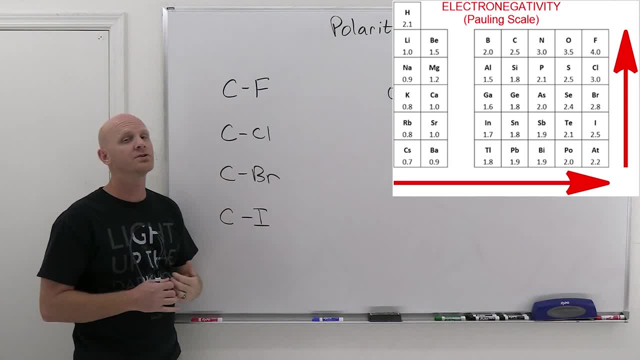 So in this case, if I said which of these four is the most polar bond, you're looking for the largest difference in electronegativity. Now, if you had, you know the Pauling scale in front of you and I'll put it up on the board here. 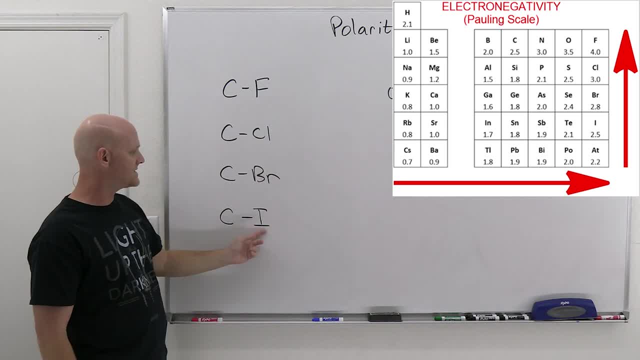 So obviously you'd see that carbon has a value of 2.5, and then iodine's at 2.5, bromine at 2.8, chlorine 3.0, and fluorine 4.0.. And so the biggest difference in electronegativity would be the carbon-fluorine bond. 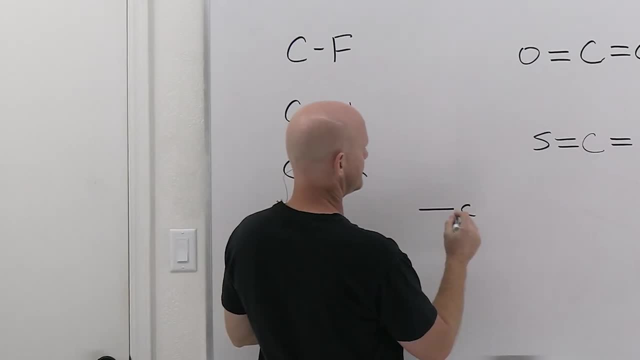 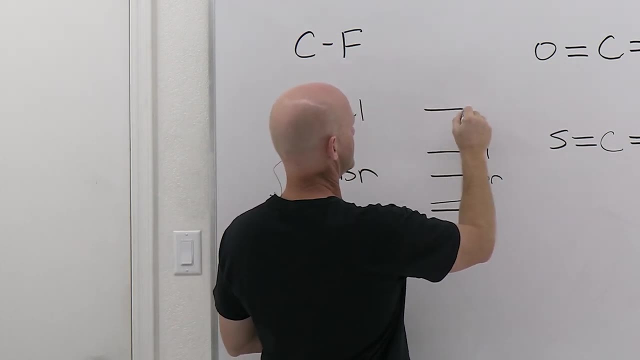 So and again you could, you know, kind of take a look at this and say: well, you know, there's carbon and iodine's almost essentially the same thing. And then you got bromine, chlorine and fluorine. 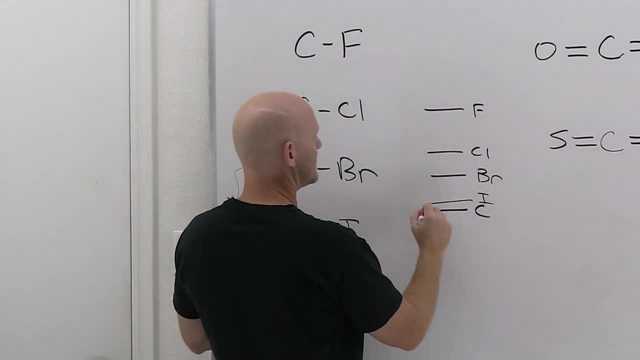 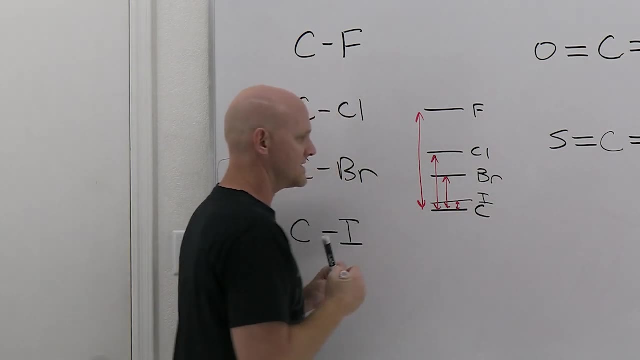 And so you're going to get your biggest difference in electronegativity between carbon and fluorine, not carbon and chlorine, not carbon and bromine, and not carbon and iodine, which have almost exactly the same value, And so identifying the most polar bonds. 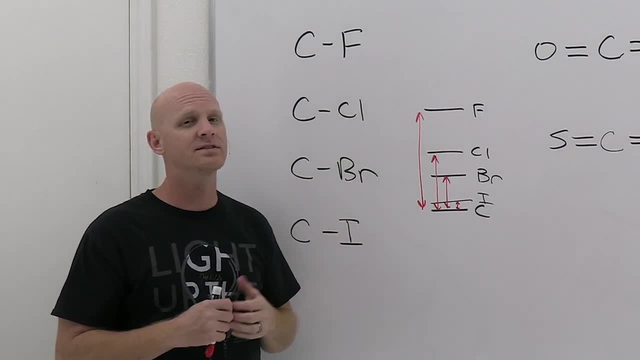 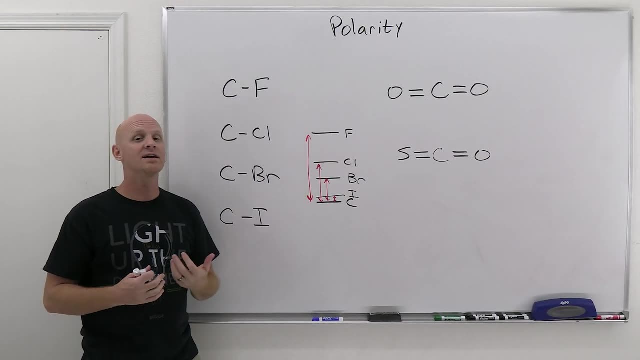 the most polar bond here would definitely be that carbon-fluorine bond, having the biggest difference in electronegativity. Now, identifying polar bonds though, here is going to be actually just the first step in now talking about identifying molecules that are polar and nonpolar. 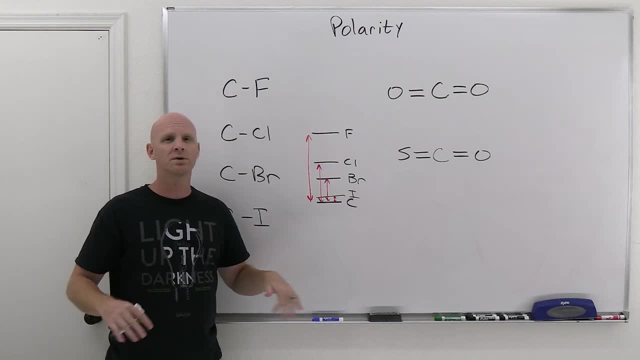 And suffice it to say this: if a molecule doesn't have any polar bonds, it is a nonpolar molecule. We'll start there, Going from there, though. if a molecule has polar bonds, it may end up being polar, it may end up being nonpolar. 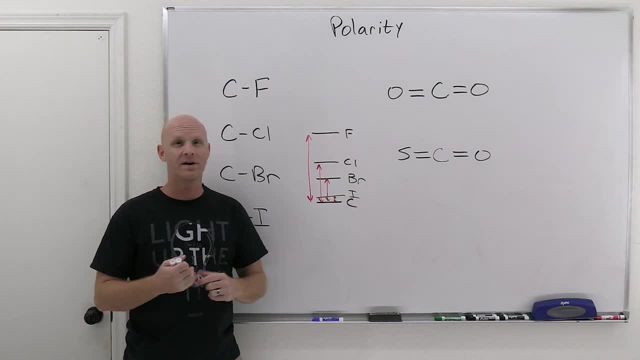 It's going to depend, And it's going to depend on what the polar bonds are and how they're oriented around the central atom. And we'll talk about if they cancel And ultimately what we mean when we say if they cancel, if the net dipole adds up to zero. 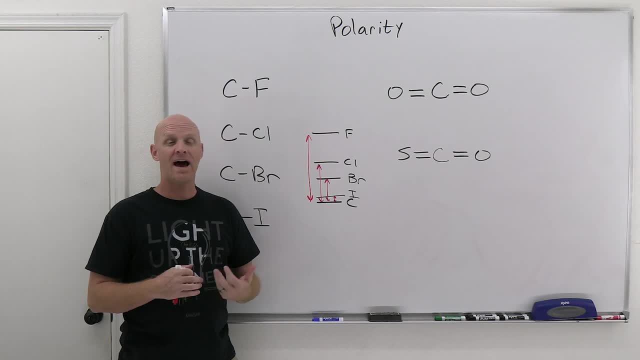 if the individual bond dipoles are oriented in such a way that adding them up as vectors sums up to zero, and we'd say a zero dipole moment, then it's going to be a nonpolar molecule, And so you've got to keep in mind what you've now learned about molecular geometry, though. 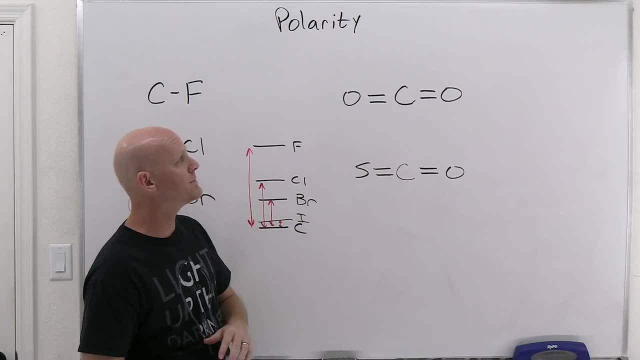 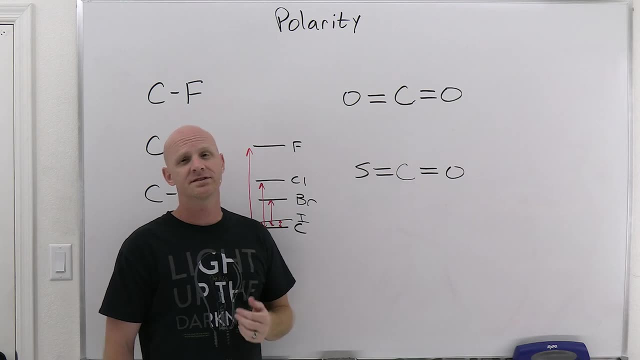 and you can't just rely on what Lewis makes things look like. Let's take a look at a couple of examples. So we'll start with carbon dioxide here, And the carbon-oxygen bonds are definitely polar. Oxygen is significantly more electronegative than carbon. 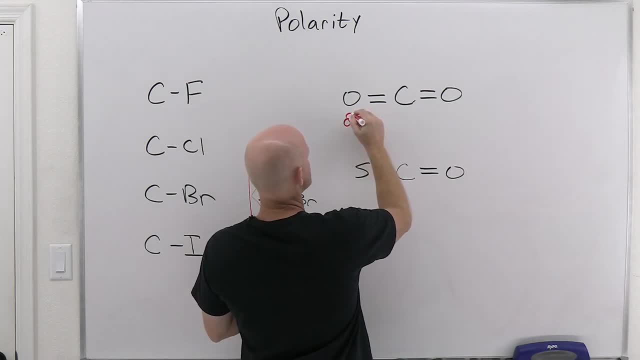 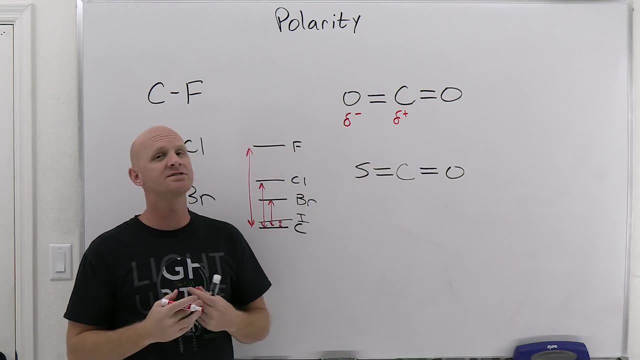 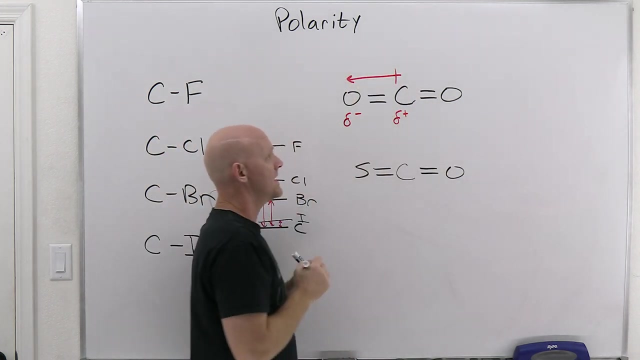 And so a couple different ways we could represent this. We could write a partial negative charge on the more electronegative oxygen and partial positive charge on the less electronegative carbon. That'd be one way to represent this polar bond. The other way is we'll often draw in a bond dipole, like so. 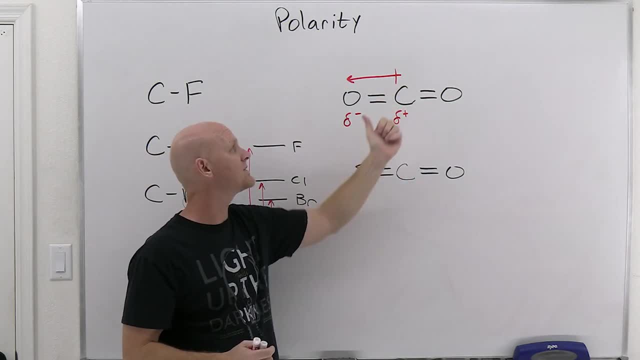 And you start with a plus sign near the partially positive, less electronegative element and then draw the arrow through towards the more electronegative, And these represent the same reality. This is just another way of showing that the carbon is partially positive. 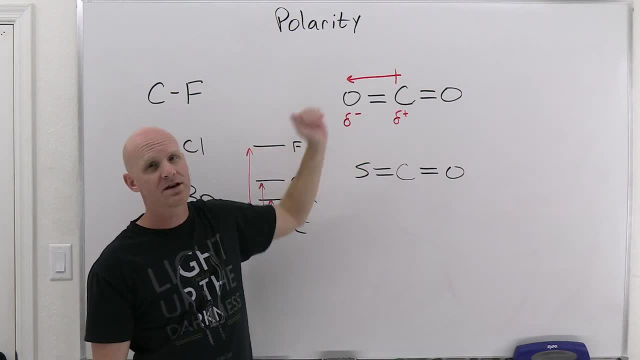 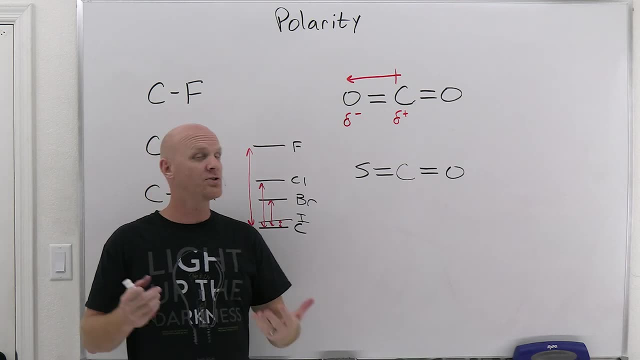 and then the oxygen partially negative. So either way you want to represent this, but this top way is often really convenient for looking at individual bond dipoles and then seeing if they either cancel or if they sum to some value and the molecule ends up being polar. 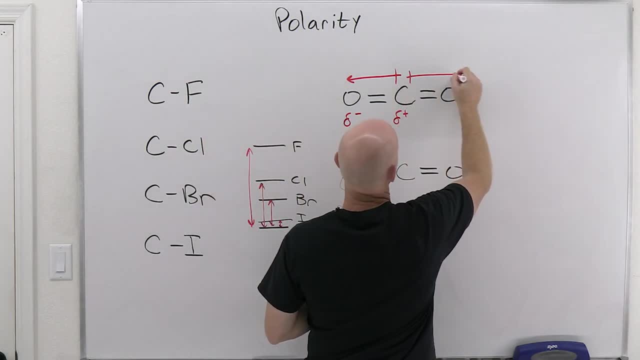 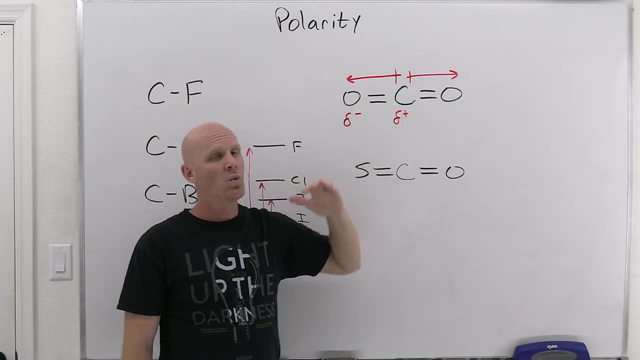 So, if we look, though, we've got another bond dipole on this side, And so in this case you've got the electrons kind of being pulled towards both oxygens here. Now, one thing you should realize here is that Mr Lewis makes these bond angles look like 180 degrees. 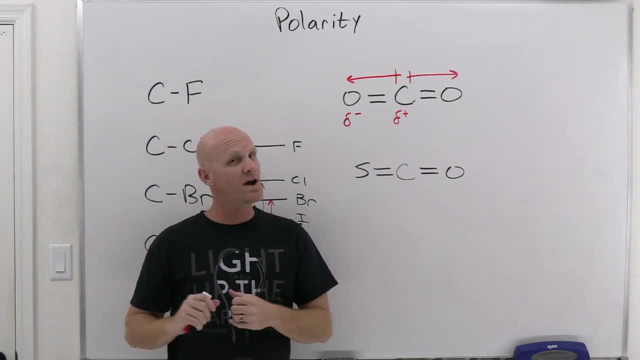 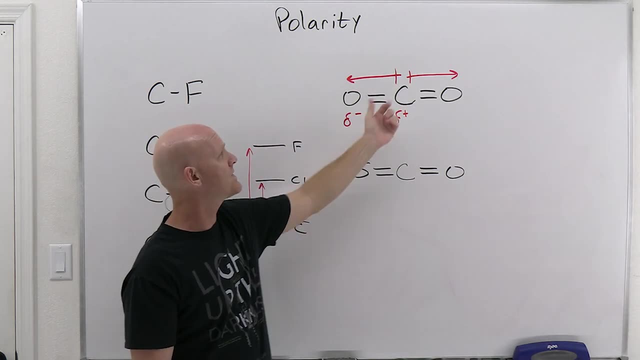 And he would be right in this case. And we'll find out, Mr Lewis is not always right, but he is right right here. So these auctions are oriented at 180 degrees apart and that's going to be important. So if we've got equal bond dipoles, since they're both carbon-oxygen double bonds- 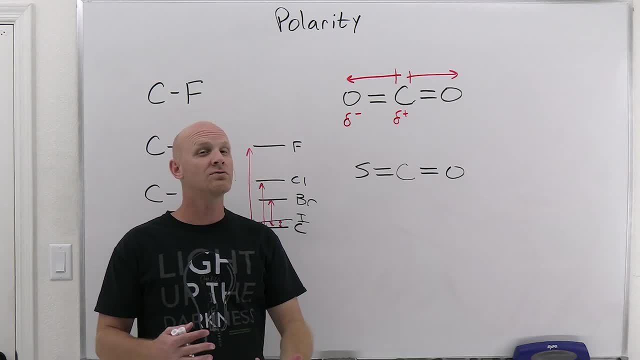 and they point 180 degrees apart. well, if you added those as vectors, they would add up to 0. And so we'd say that this molecule, even though it has individually polar bonds, overall it has no overall dipole or no dipole moment. we might say. 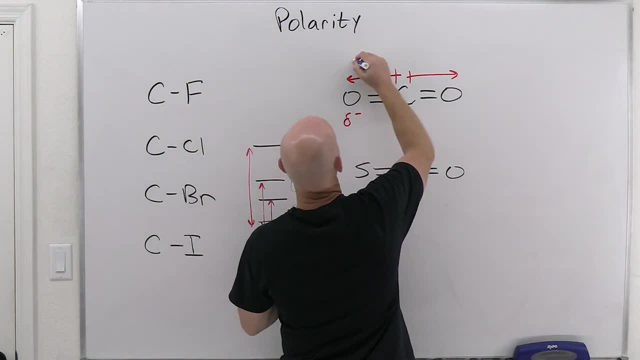 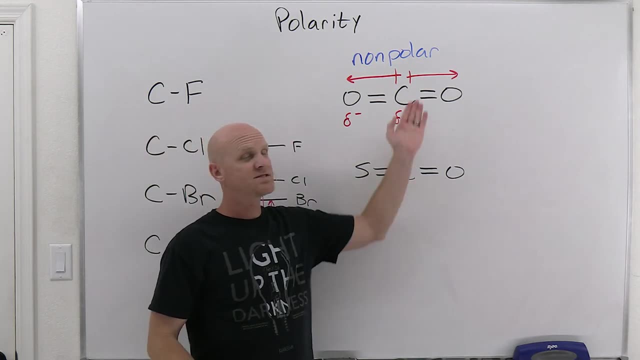 And, as a result, we'd say that this molecule is nonpolar. So oftentimes we'll explain this to students And instead of looking at this as the sum of vectors- because that's usually something you'll study in more detail in physics- 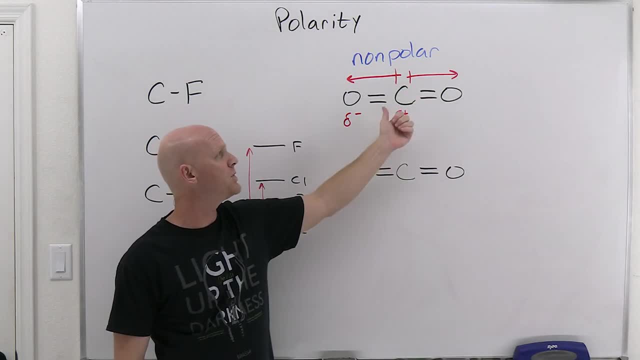 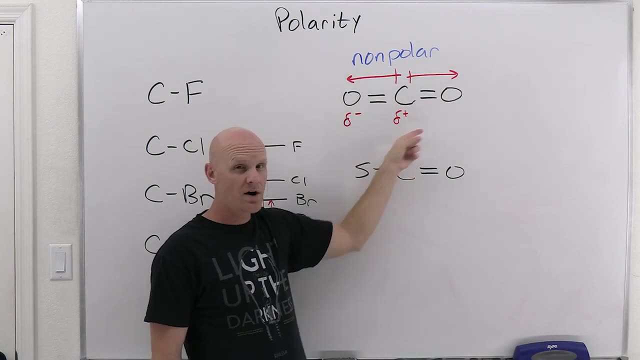 and a lot of our students haven't had physics yet. we might talk about, you know, pulling a rope on this, this carbon, And if we pull equally- since these are both auctions equally in exactly opposite directions, since the bond angles are 180 degrees. 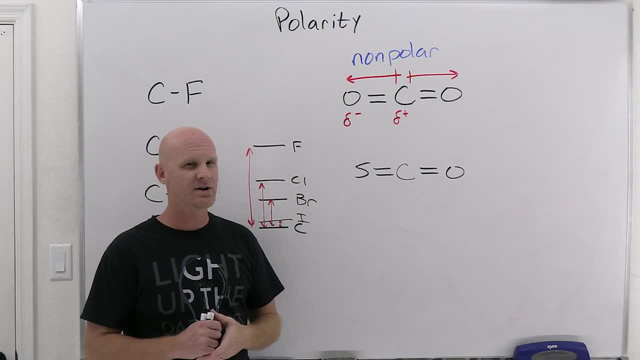 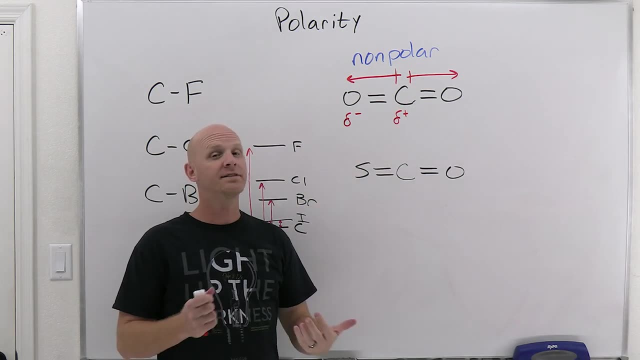 the question is: would the carbon go anywhere? It's kind of how we like to phrase this. In this case, it wouldn't. If they're pulling equally in exactly opposite directions, well then the carbon is not going to be pulled net in any particular direction. 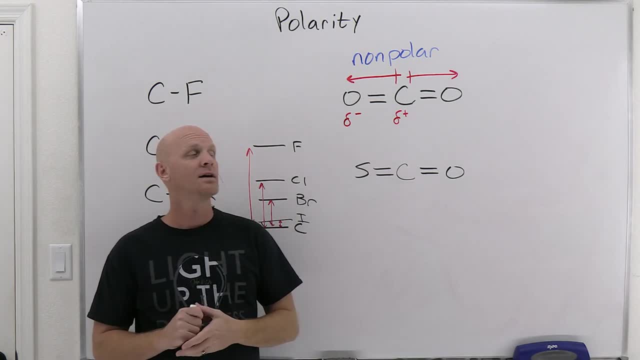 And that's one way of giving you know, getting evidence, that the bond dipoles add up to 0, and the overall dipole moment is 0. So the molecule is nonpolar. If you get a 0 dipole moment, you're nonpolar. 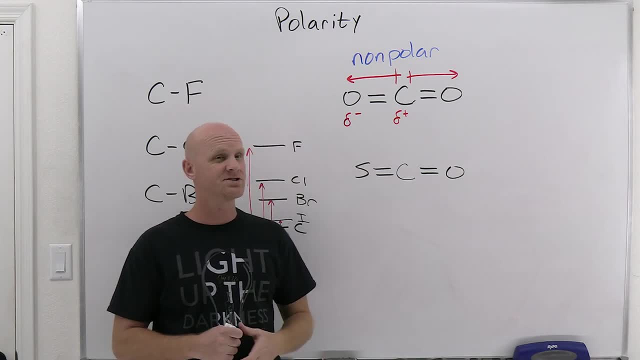 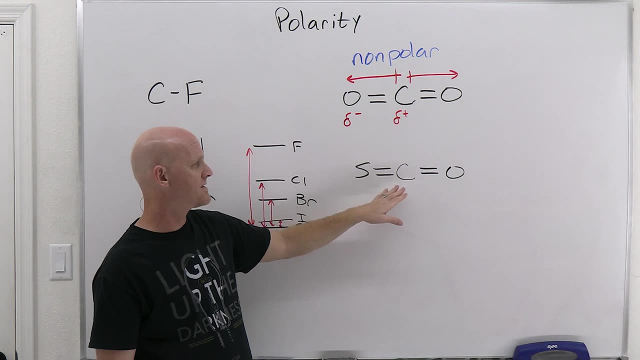 If you get a non-0 dipole moment, then you're polar. is generally how this works, And the greater the dipole moment, the more polar the molecule. So if we contrast that with this lovely molecule here, where we replace one of the auctions in carbon dioxide here with a sulfur, 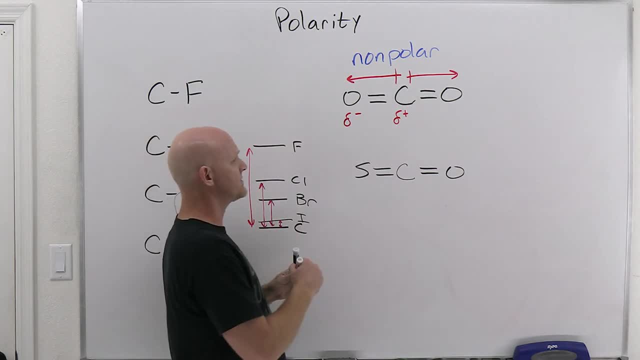 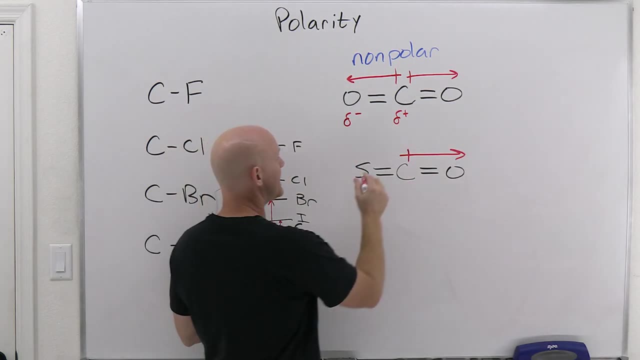 one row down on the periodic table, one period down. So we've still got two polar bonds here. The carbon-auction bond, again still polar. The carbon-sulfur bond is a little bit polar, but much less than the carbon-auction bond. 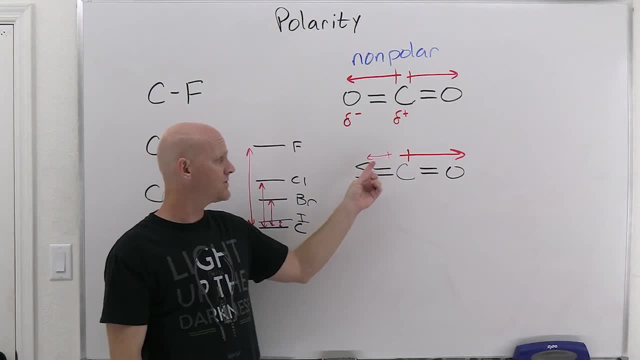 And so I'm going to draw a smaller arrow, And as a result, we still have two bond dipoles that point 180 degrees apart, but they're not equal in magnitude, And so they don't add up to 0 this time. 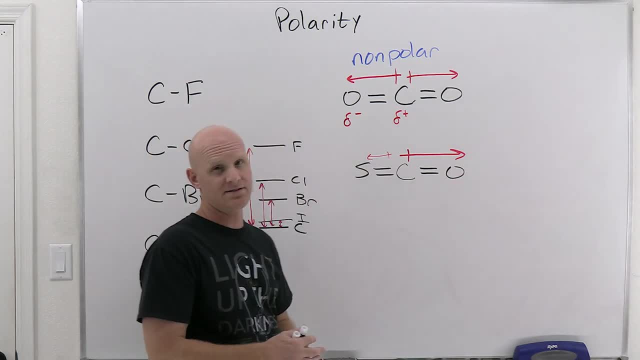 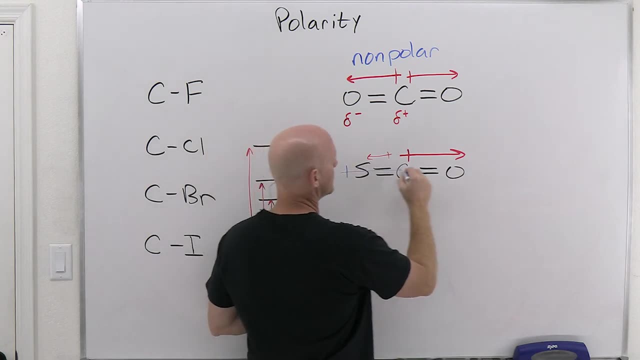 And so overall, we're going to have an overall dipole moment pointing towards the right. And so when you have an overall dipole moment, sometimes they have you draw those in And in this case the overall molecular dipole would point to the right. 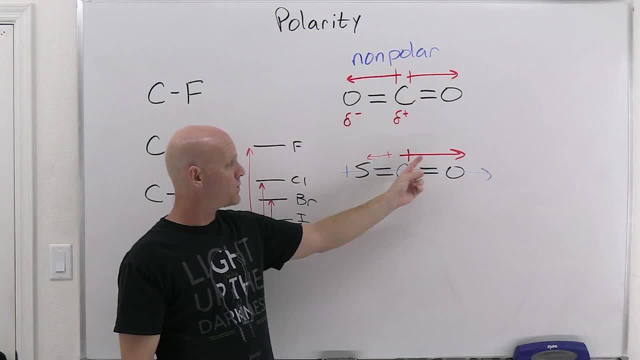 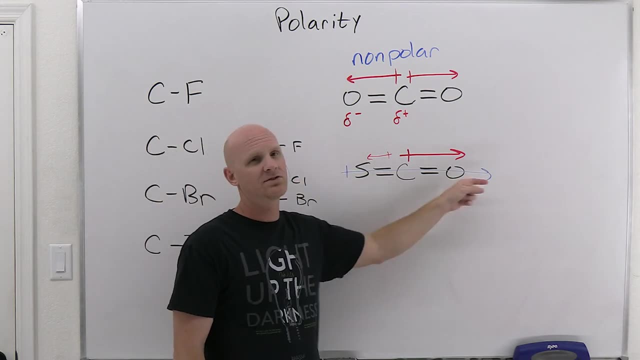 because, essentially, adding this bond dipole with this one, the one pointing to the right, is more than going to make up for the one point of the left and then some, And so the overall molecular dipole is going to point towards the right, And so, in this case, 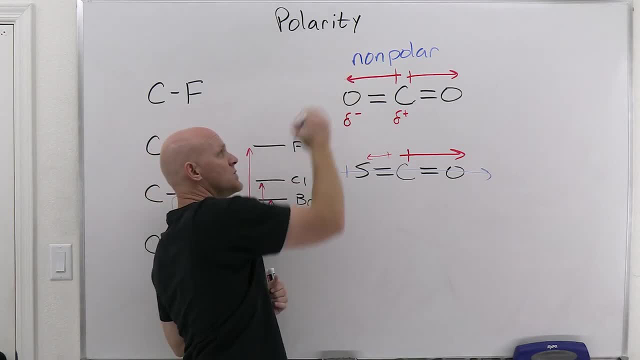 both these molecules have polar bonds, But whereas the first one, the individual bond dipoles canceled, it was non-polar. in the second one they don't completely cancel, And so we refer to this molecule as being polar, And so we've kind of learned the strategy, then, for identifying molecules. 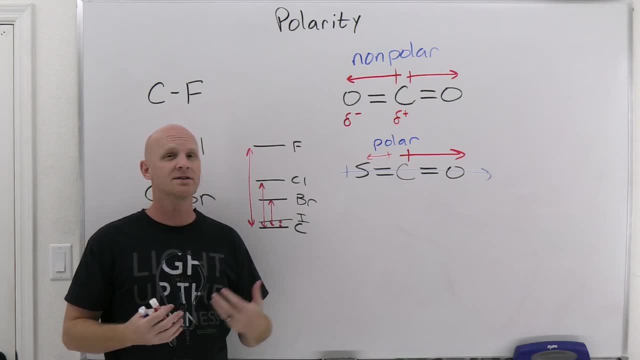 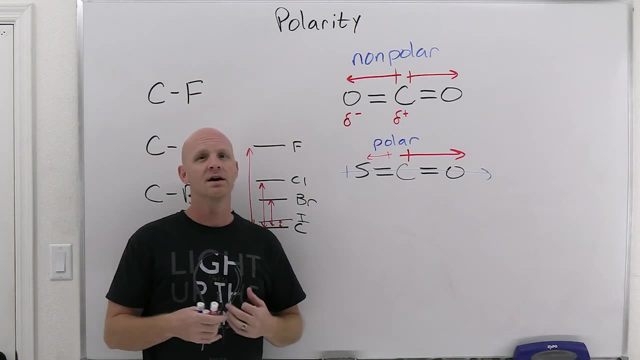 as being polar and non-polar, And it turns out this is really important because it turns out this is going to affect the properties of these molecules and things like boiling points and melting points and viscosity and things of a sort that we're going to study later on. 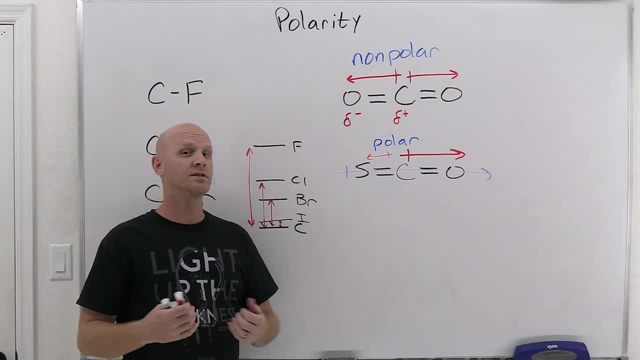 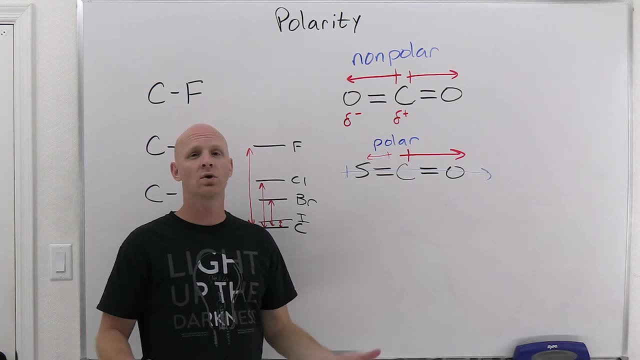 So it's actually rather important to the properties of a material whether or not you can identify it as being polar and, in some cases, how polar. So but first thing you want to do then in the strategy is just identify. do you have any polar bonds? 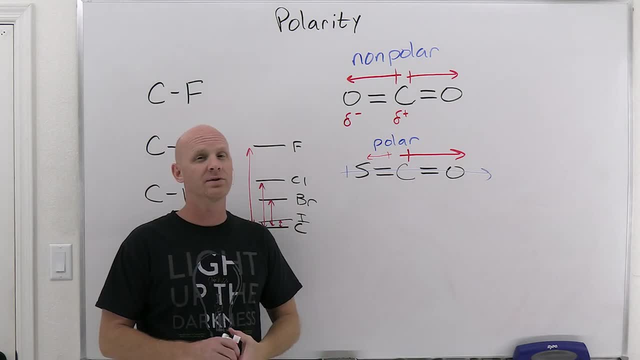 If you say no, then no. polar bonds means it's going to be a non-polar molecule. But if you have polar bonds, then you got to look at how they're oriented and their magnitudes and say: do they cancel, ie do they add up to a net dipole of zero? 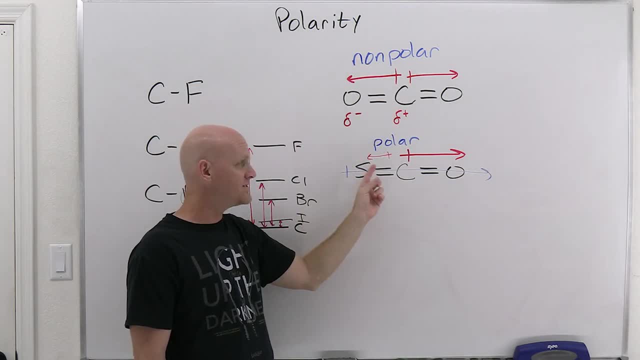 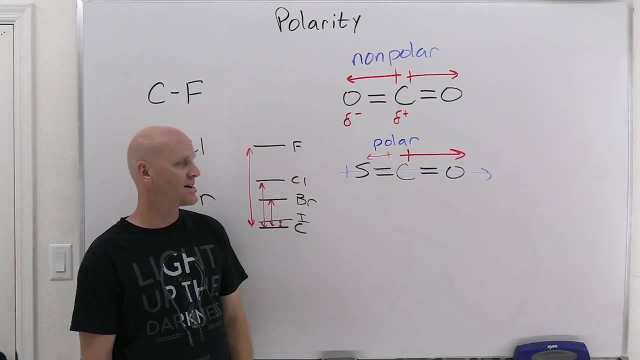 If they add up to zero and cancel, then it's a non-polar molecule. If they don't perfectly cancel, then it's still going to be, have some residual polarity and be a polar molecule, as in the second case here. So one thing you got to be careful of is you got to be careful of Mr. 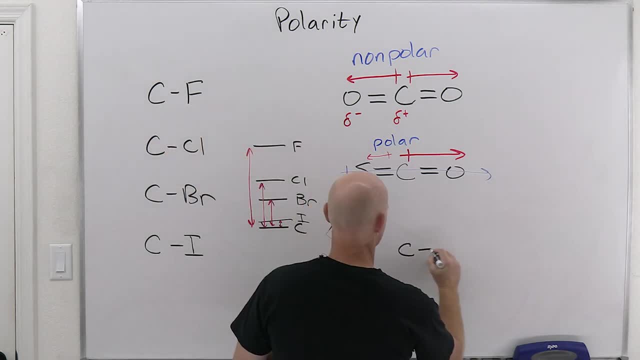 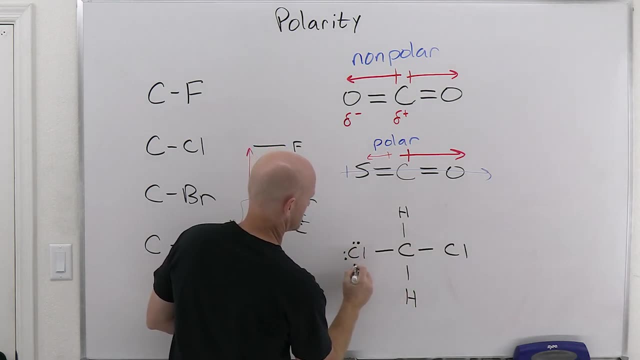 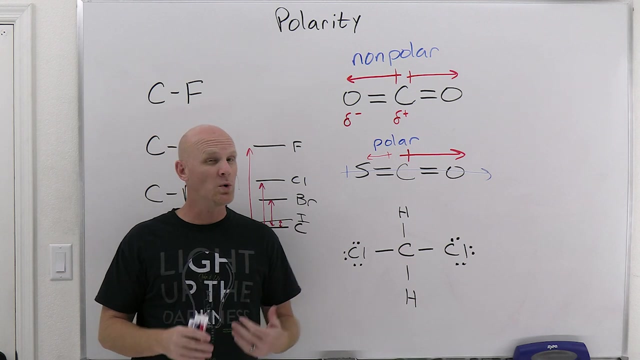 Lewis, because he doesn't always tell the truth. So if we take a look at this example here, So here's CH2Cl2.. And this molecule is indeed polar, as we're going to find out, but it's really common for students to assign this one as being non-polar. 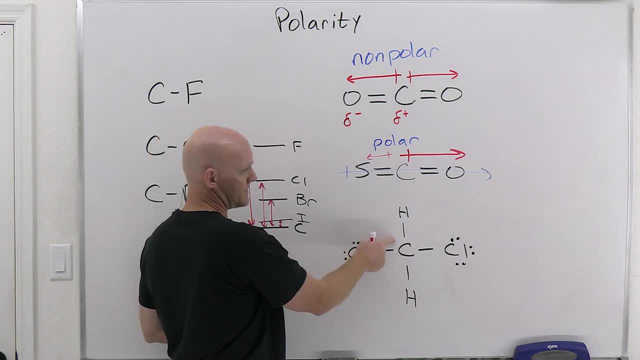 because they look at this and they're like: oh, let's see, We were told, Chad told us, you know that carbon-hydrin are the two different atoms that still form a non-polar bond, And that's true. 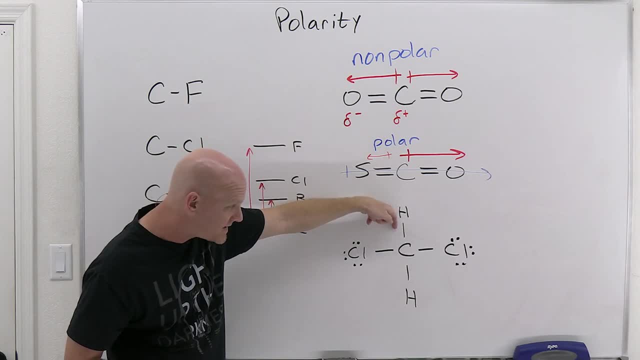 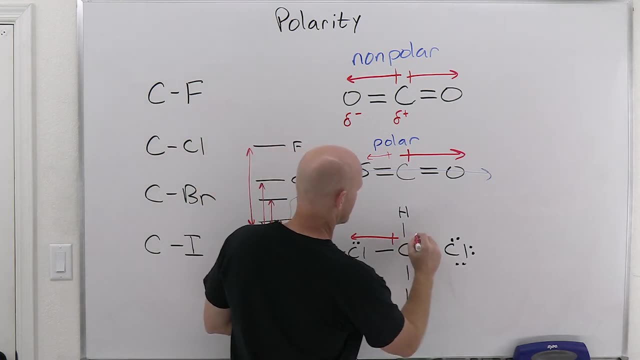 Turns out, carbon is just slightly more electronegative and technically you'd have a really tiny bond dipole pointing towards the carbon that you can pretty much ignore. But the carbon-chlorine bonds are indeed polar, And so a lot of students look at this and they're like: 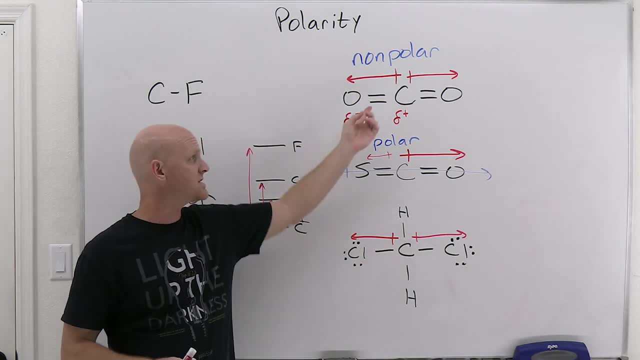 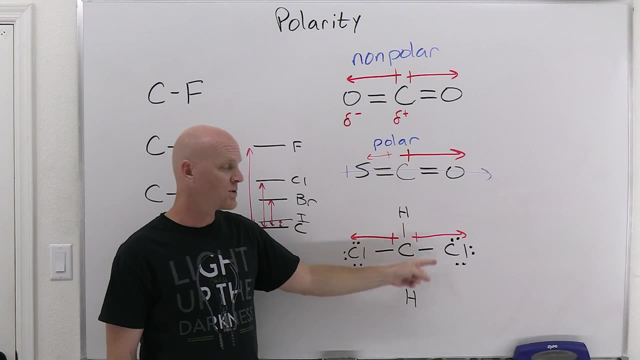 oh, they're equal in magnitude. They're 180 degrees apart, And so, yeah, it's just like CO2 and this is non-polar. Except the problem is is that they're not 180 degrees apart. So carbon, here's got four electron domains. 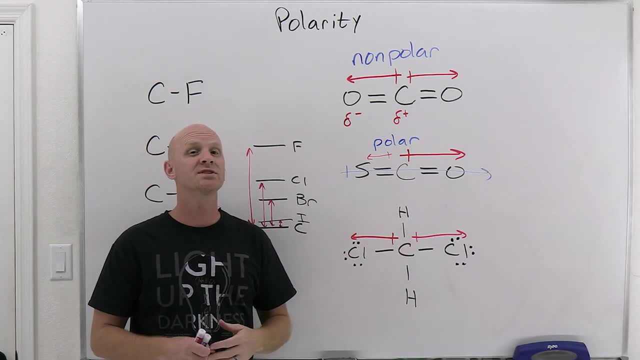 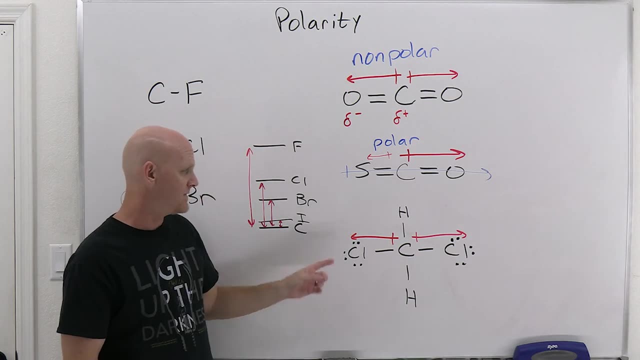 and with four electron domains, you're supposed to know that the electron domain, geometry is tetrahedral and the bond angles are not 180.. They're 109.5.. And so, even though, again, Mr Lewis makes everything look either 90 degrees or 180 degrees, 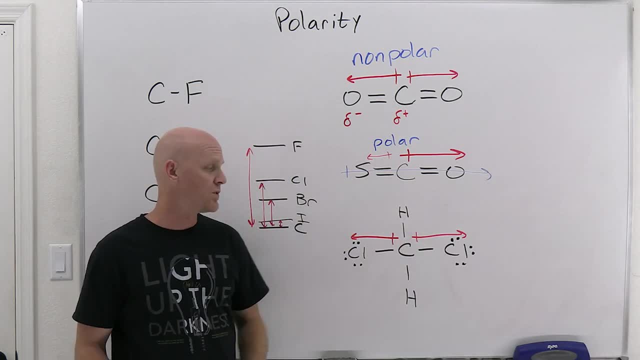 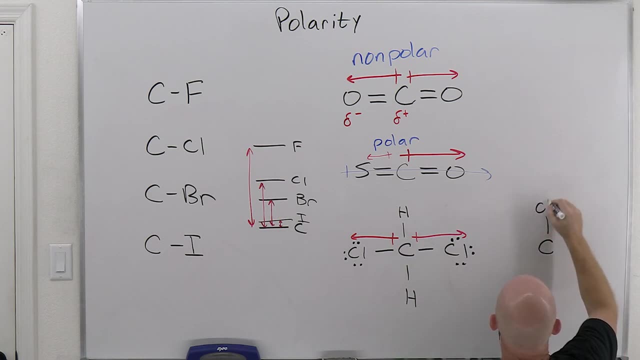 none of the angles in this molecule are 90 or 180.. They're all 109.5.. And so if we try to draw a little better three-dimensional representation of this molecule, we can kind of see what's going on. And so here we kind of represent that tetrahedral structure here with four electron domains. 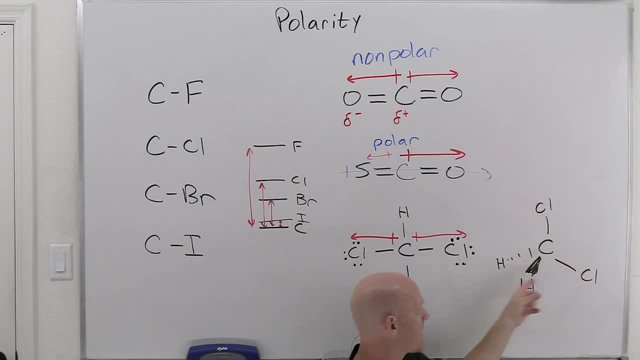 and kind of see the bottom of the pyramid right here and then going up to the chlorine for the top of the pyramid. And if now we draw in those polar bonds again, one here and one here, we can now see that these don't point 180 degrees apart. 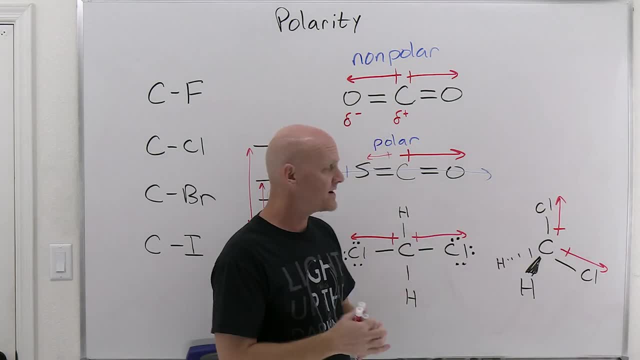 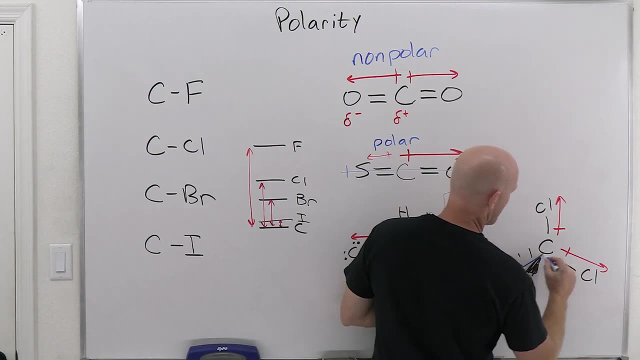 They're just 109.5 apart and they're not going to cancel. And in fact when you add those two together as vectors, you get the average of them, and the average of them would point right down the middle of this molecule. And so the overall molecular dipole moment is what I've diagrammed in blue. 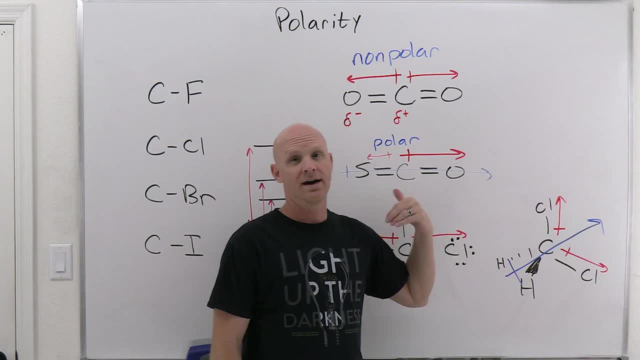 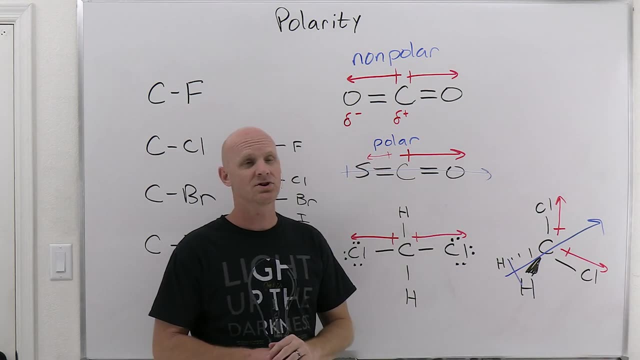 It's when you again sum up all the individual bond dipoles And again, if they don't cancel perfectly, then you're going to have some overall molecular dipole that you could potentially draw in like we've done. so Cool, And so, once again, this molecule is indeed polar. 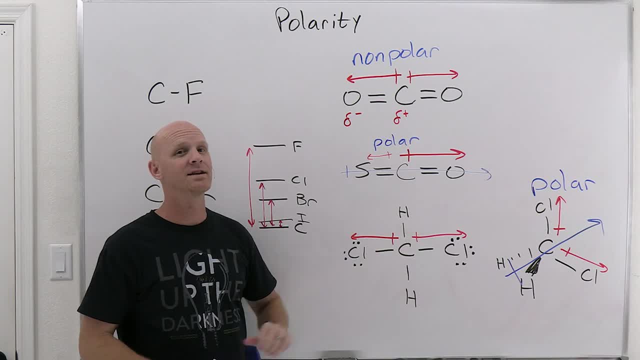 But again, drawing the Lewis structure like this, a lot of students would mistakenly identified as being nonpolar. But no, no, definitely polar. Don't make this mistake. Now one thing to note here, if you've noticed in the first example, 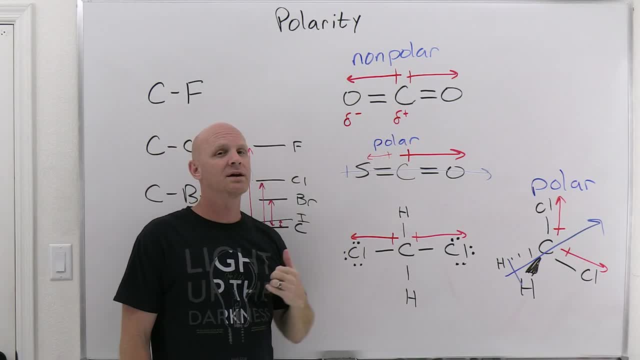 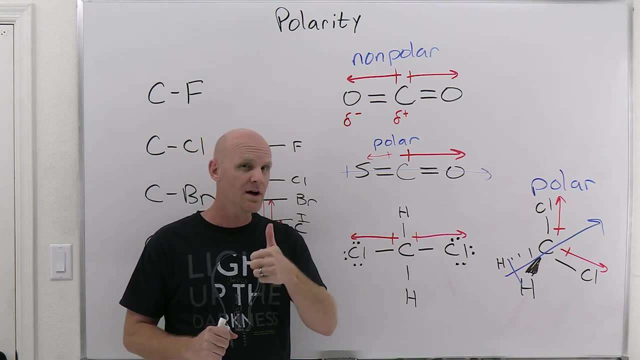 we had two of the same atom around the central atom and it ended up being nonpolar. Now, sometimes that'll end up being polar, sometimes nonpolar, And we'll see that lone pairs around the center. We're going to be something really important to identify here in a second. 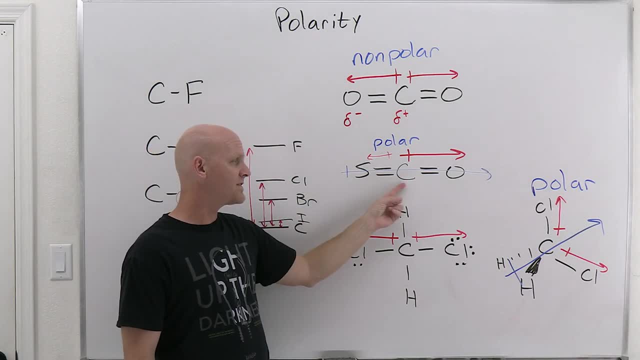 But in these last two examples, when we had different atoms around the central atom, different atoms around the central atom, usually the case is that's going to end up being polar, because your individual bond dipoles are not usually going to cancel. That's another thing to identify. 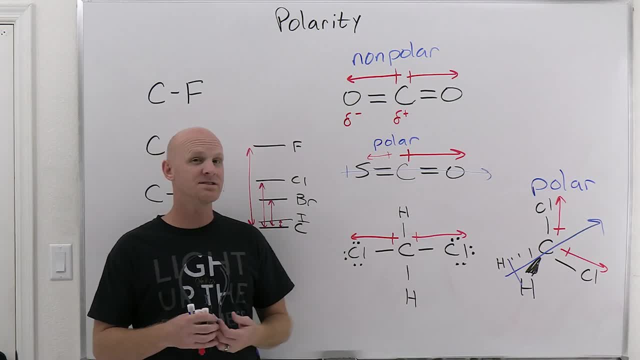 But most of the molecules are actually going to be, you know, asked to identify as being either polar or nonpolar. They're going to have identical atoms all the way around and we'll have a pattern to recognize for identifying these as polar or nonpolar. 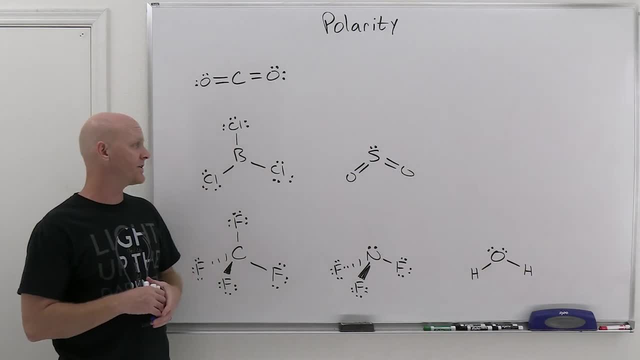 Here that we'll take a look at. So now we'll take a look at some more examples here, and I just want to point out the first three. and obviously we already did carbon dioxide, So. but what you're going to notice is that if you've got all of identical atoms around the central atom, 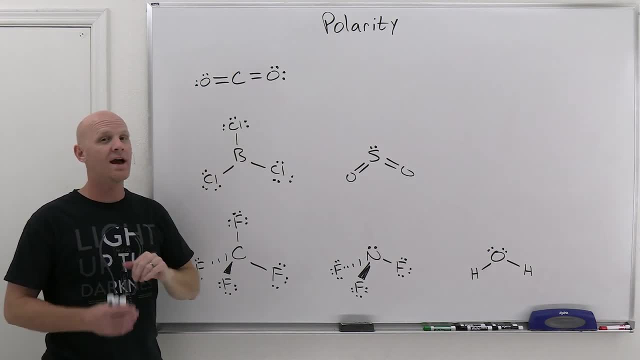 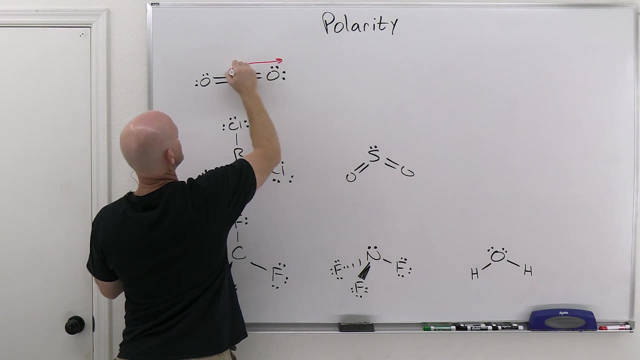 and that central atom has no lone pairs, then your bond dipoles will cancel and it will be nonpolar. So, and again we saw that with carbon dioxide, These really were oriented 180 degrees apart and the bond dipoles cancel, adding up to zero again, making this nonpolar. 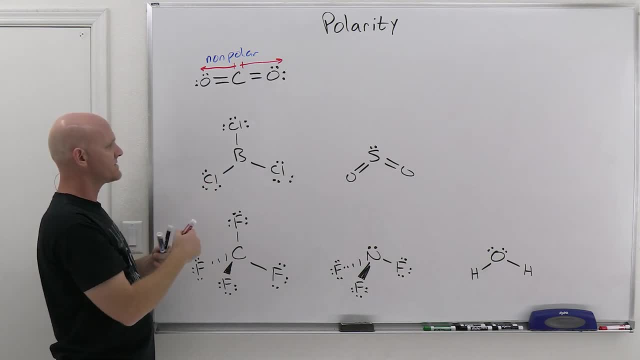 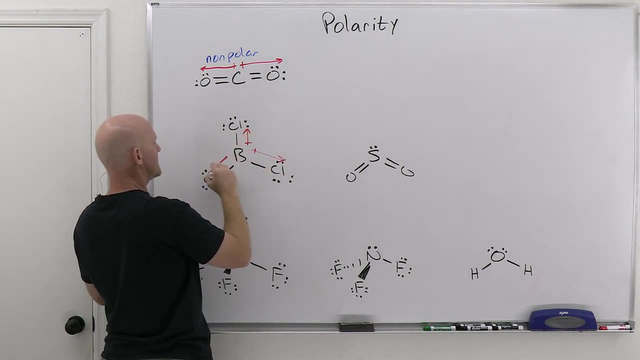 Having a zero dipole moment Now in the case of BCL3.. So this guy's trigonal planar and your bond dipoles here are all oriented 120 degrees apart And if you pulled on this boron in three different directions. 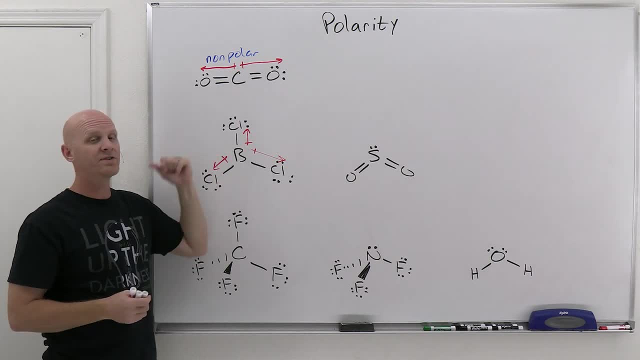 120 degrees apart, he'd go nowhere. All these bond dipoles add up to a vector sum of zero. And again he ends up being nonpolar. And again it's important to recognize that. again, Lewis doesn't always tell the truth. 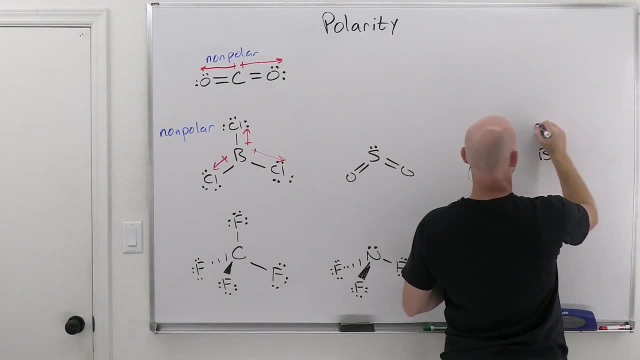 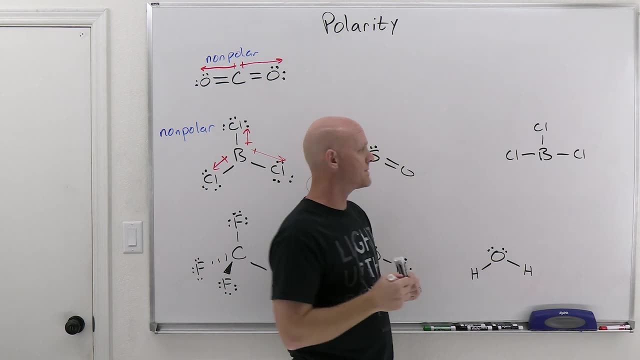 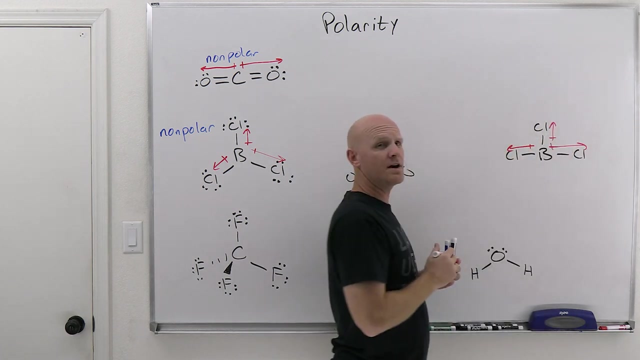 Because we commonly would draw the Lewis structure for this guy So like so. and if you draw the Lewis structure like this, making everything look 90 or 180 apart, and you draw in those individual bond dipoles, you might be like, well, these two cancel, but nobody cancels him out. 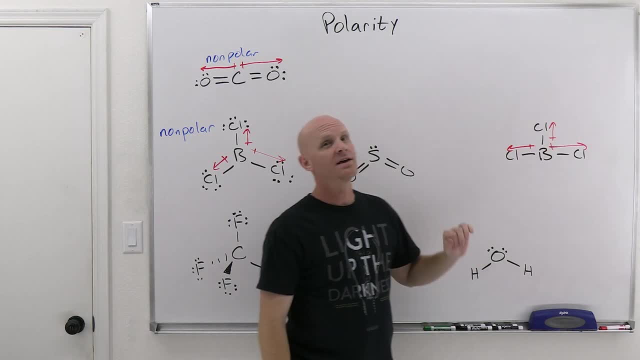 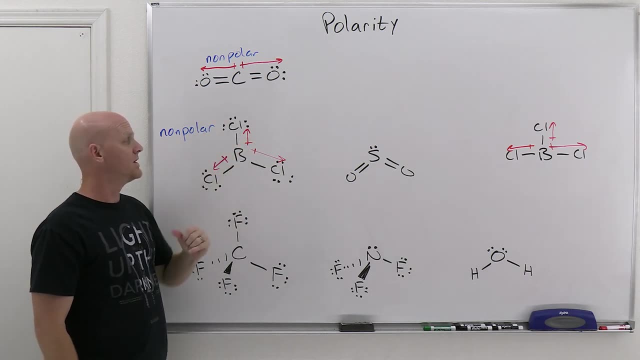 But again, you have to remember that don't go by what Lewis tells you the angles are. You have to know, based on your knowledge of molecular geometry. Now, what are the real bond angles, What is the real three-dimensional geometry Or, in this case, two-dimensional geometry? 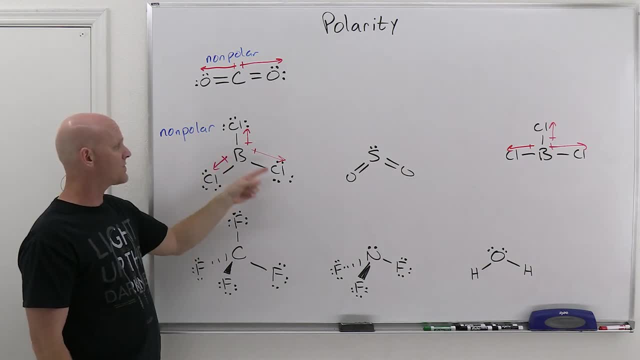 What does the geometry of this guy look like? Well, he's trigonal planar with three electron domains, And these are all 120 degrees apart, Not either 90 or 180 apart, like Lewis might make you think. And so, again, don't just rely on what the Lewis structure looks like. 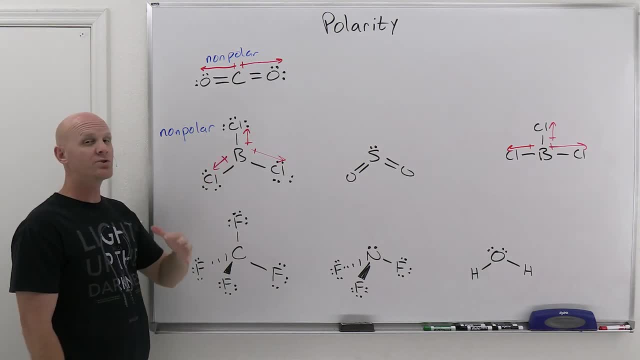 Keep in mind what is the actual molecular geometry look like when you're trying to figure this out. Same thing here. We'll move on to CF4. here In CF4, we've got four electron domains, So therefore it's going to have an electron domain geometry that is tetrahedral. 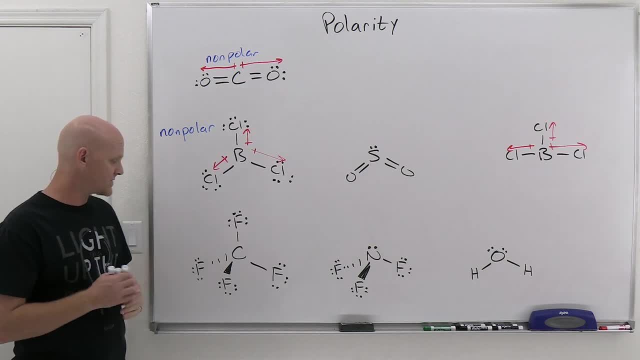 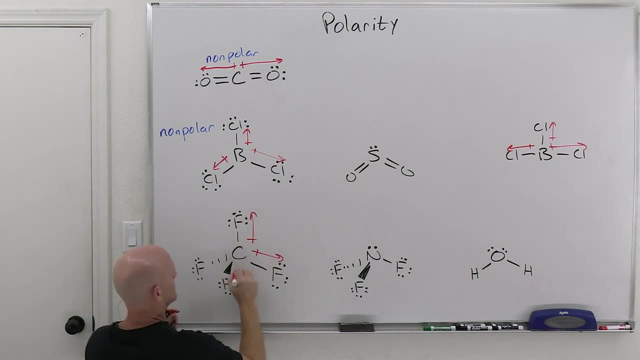 And with all of them being bonding, that means the molecular geometry is also tetrahedral, And so all these bond angles are 109.5.. And again, they're all equal in magnitude, since they're all carbon-fluorine bonds. 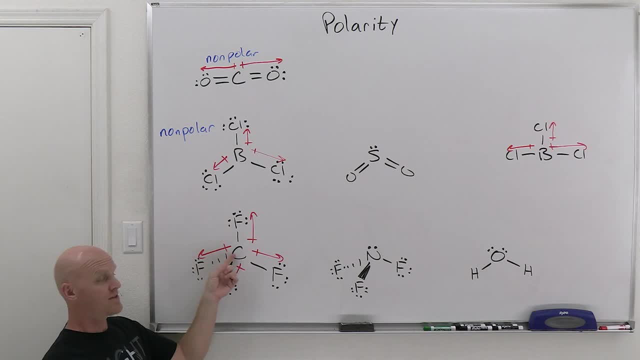 And they're all oriented 109.5 degrees apart And it turns out they're going to add up to a vector sum of zero, And this one is not so easy necessarily to visualize, with it being three-dimensional and stuff, But trust me it will add up to zero. 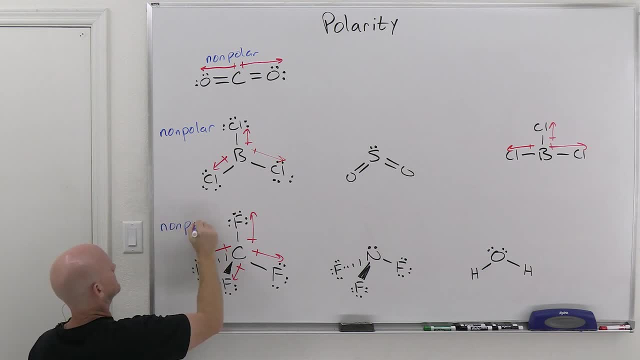 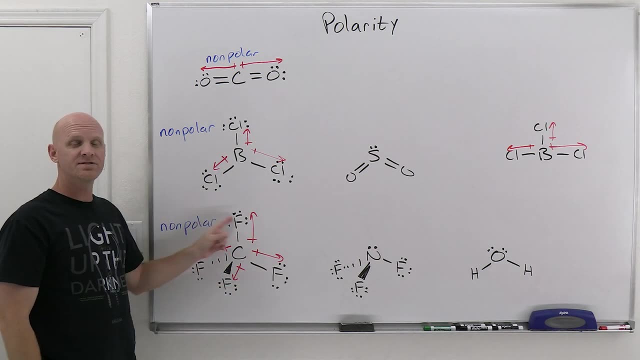 And this guy is also nonpolar. And, once again, if you have identical atoms all the way around your central atom and no lone pairs on the central atom, it will be a nonpolar molecule. rest assured, That's something you can take to the bank. 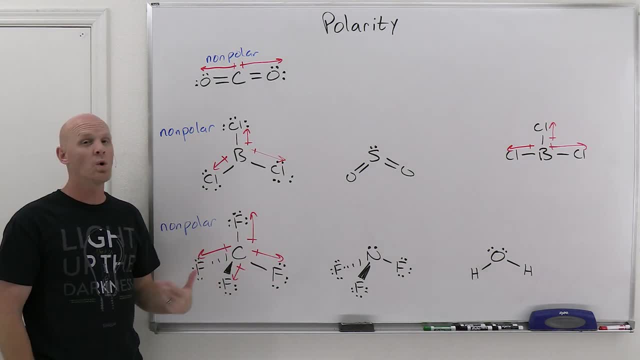 Now, if I replace a couple of these fluorines with a couple of hydrogens, or even one of these fluorines with a hydrogen, or three out of the four fluorines with three hydrogens, or something like that, well then I wouldn't have the same atoms all around. 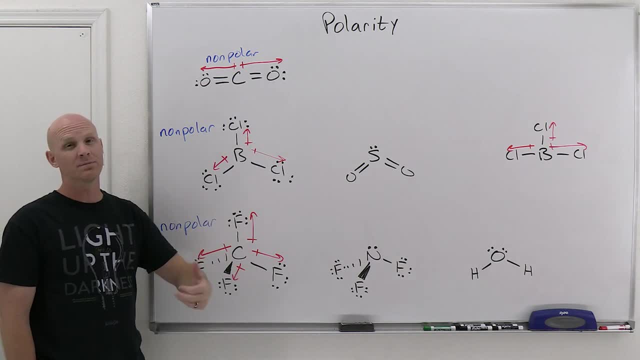 and it wouldn't necessarily have bond dipoles that cancel. Then it would end up being polar. But again, for now we're just going to consider several examples where all the outside atoms are identical. Now let's see what happens when we put lone pairs on the central atom here. 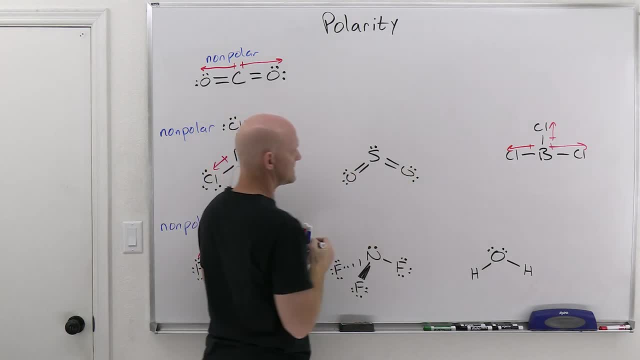 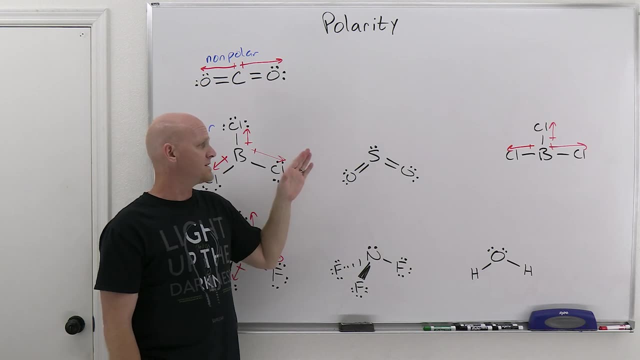 And I forgot them off- the outside atoms. But in these next two examples the central atom is going to have a lone pair in both of these. Now for the first one, here with SO2, so sulfur here has got three electron domains. 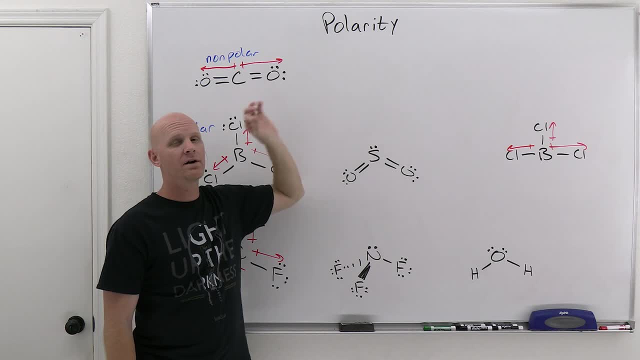 Two of them are bonding. It's bonded to two atoms and a lone pair With three electron domains. that electron domain geometry is going to be trigonal planar, But with a lone pair on the central atom. the molecular geometry will not have the same name. 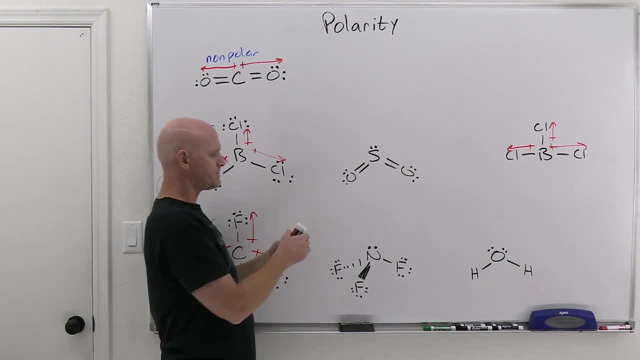 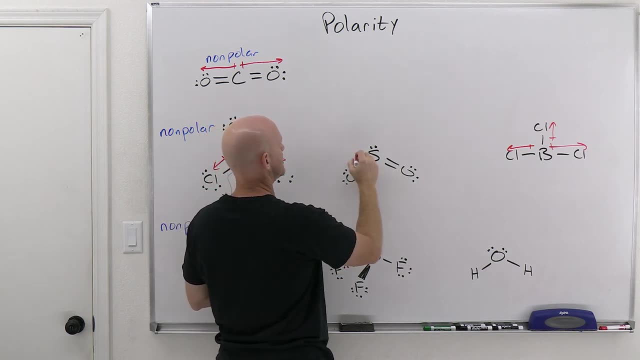 but in this case will be bent, And so I've drawn the kind of the three-dimensional geometry here. These are not 180 apart, They're closer to 120 apart, And if we draw in those bond dipoles, knowing that they're about 120 apart, 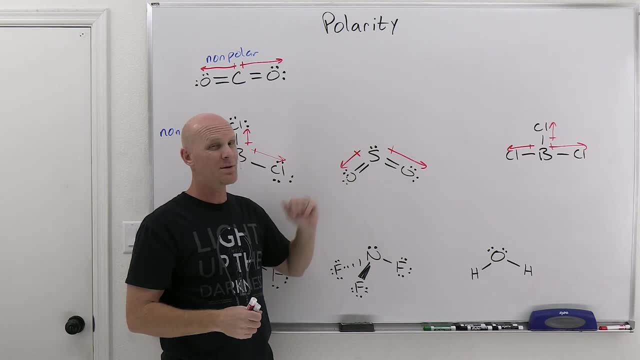 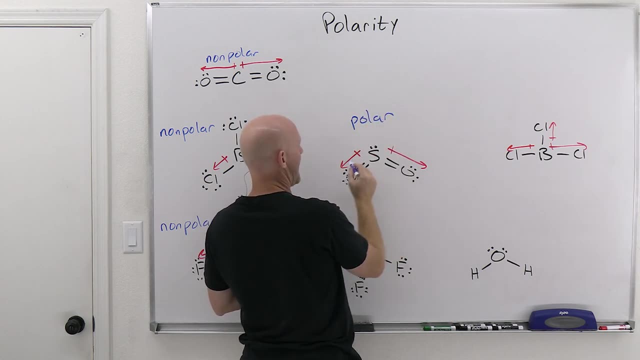 well, in this case, since they're not 180,, they are equal in magnitude, But since they're not 180 apart, they're not going to cancel perfectly, And this guy is indeed going to be polar And the average of these two bond dipoles. 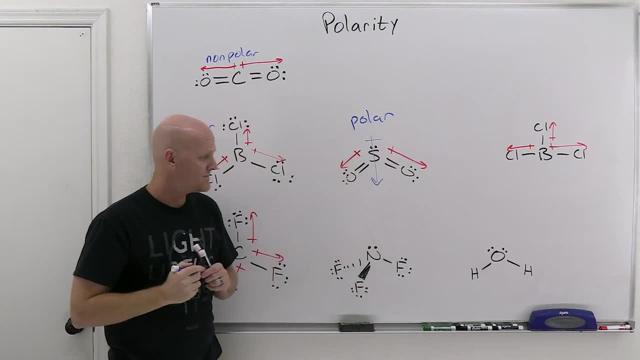 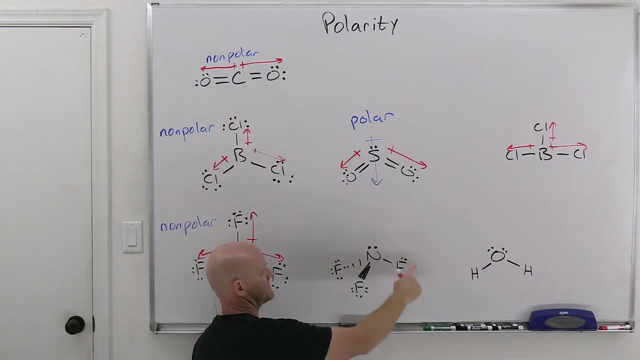 would be a bond dipole pointing right down the middle of that molecule. We'll see something similar here with NF3. And once again we've got three polar bonds, So those NF bonds, And we could draw in those individual bond dipoles. 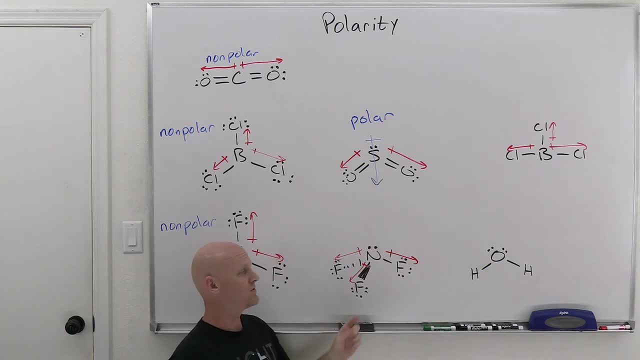 But once again that central atom's got a nitrogen on it. So keep in mind, nitrogen here has got four electron domains, So three that are bonding and then one lone pair of electrons. So that's going to make his electron domain geometry tetrahedral. 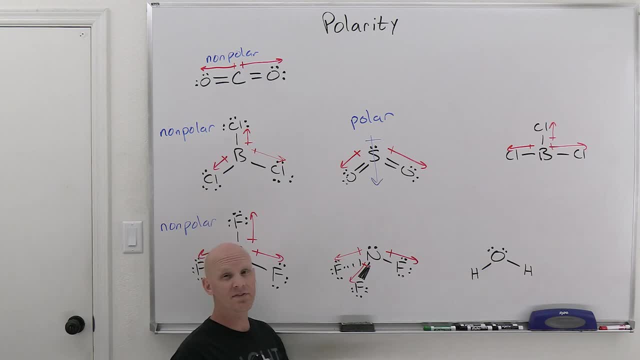 But again, with the central atom having a lone pair, the molecular geometry will not get the same name, In this case with three bonding domains and one lone pair. it's called trigonal pyramidal, you might recall, But the angles here are all roughly 109.5. 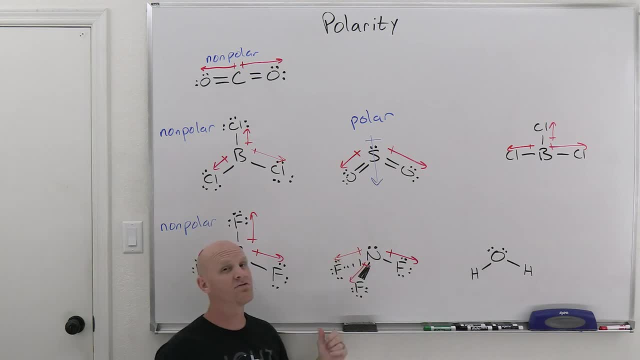 Keep that in mind. And so in this case, if the nitrogen had been surrounded by four fluorines, like carbon had over here with another one pointing up, they would have canceled. But without the fluorine up top pointing up, these three aren't all perfectly going to cancel. 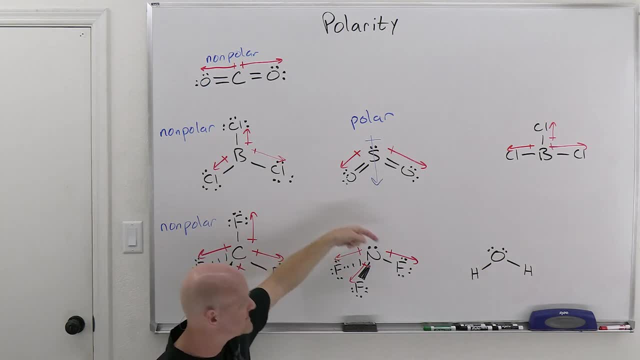 In one way, shape or form, they all are pointing downward And, as a result, right down the middle of this molecule there's an overall bond dipole And this molecule, this molecule, is polar. Those bond dipoles don't perfectly cancel. 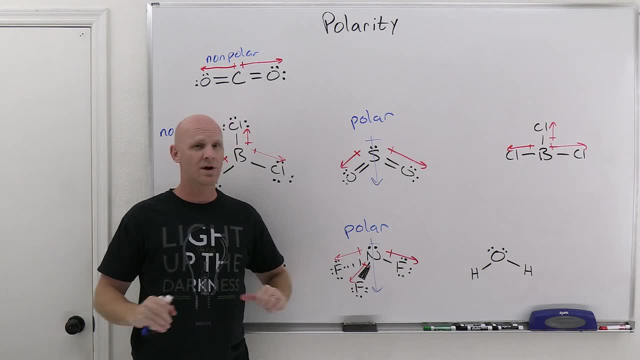 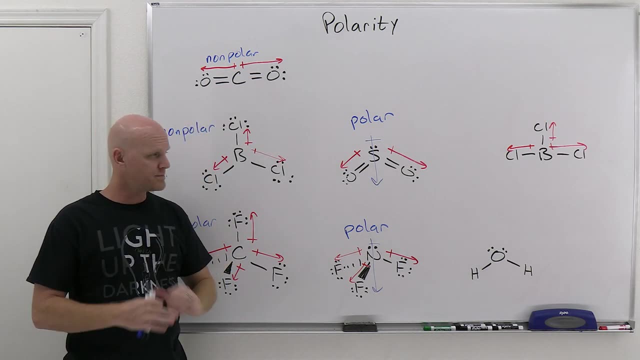 And so again, here's the deal Again, assuming you have all identical atoms around the central atom. we've now taught you that if there's no lone pairs on the central atom, it will be nonpolar. All the bond dipoles will cancel. 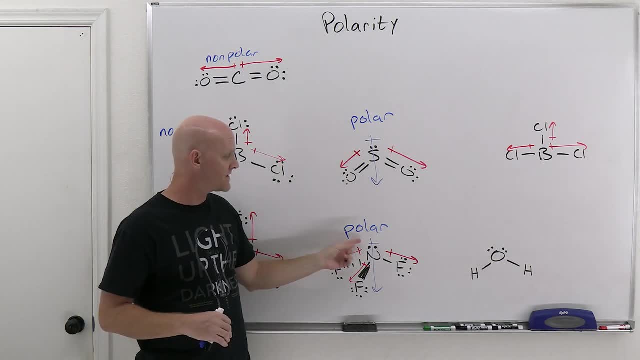 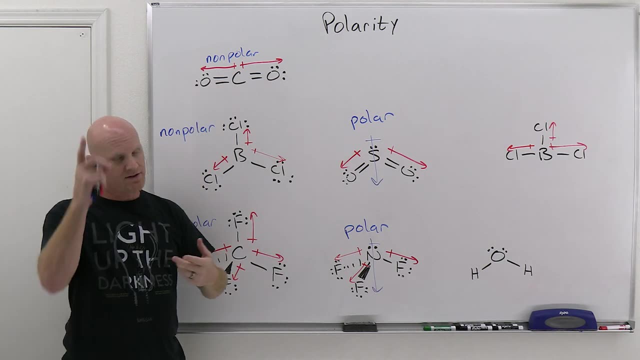 Cool. And now we've shown you two examples where there's lone pairs on the central atom and they both ended up polar. And so students get to thinking that well, if there's no lone pairs in the central atom, and again assuming all identical atoms all the way around, 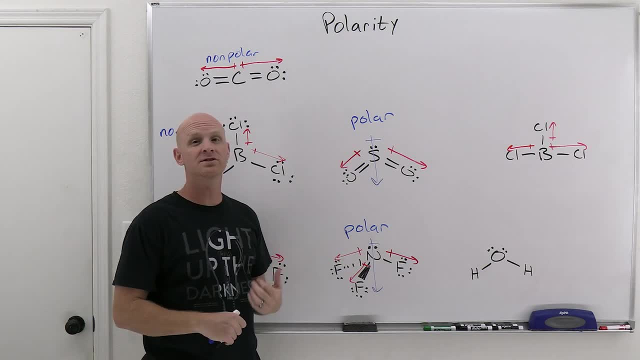 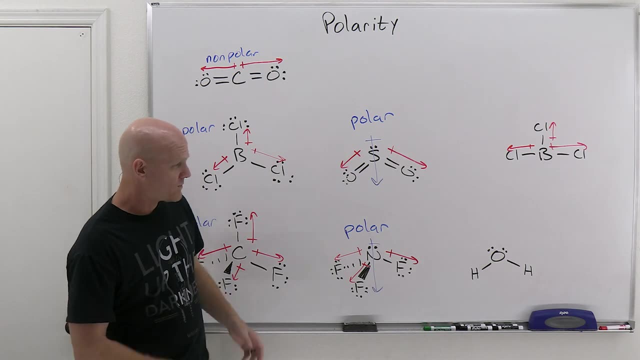 it's going to be nonpolar, And if there's lone pairs on the central atom it's going to be polar, And most of the time that would be correct. So, but you've got to be a little careful. So let's look at one more here, with water that you're commonly going to see. 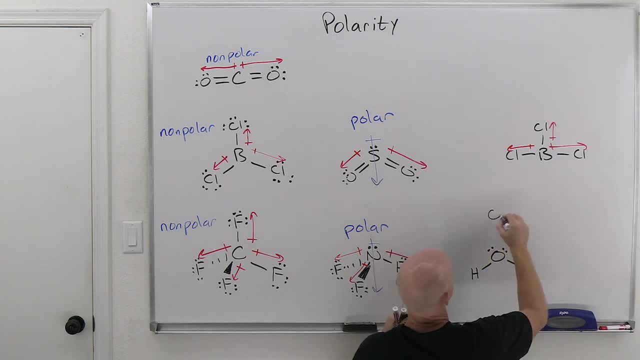 And again it's another one. that's a little bit tricky because the Lewis structure is often drawn like so, And if you just go by what Mr Lewis says, these look like they're 180 degrees apart. and they're not. They're again. 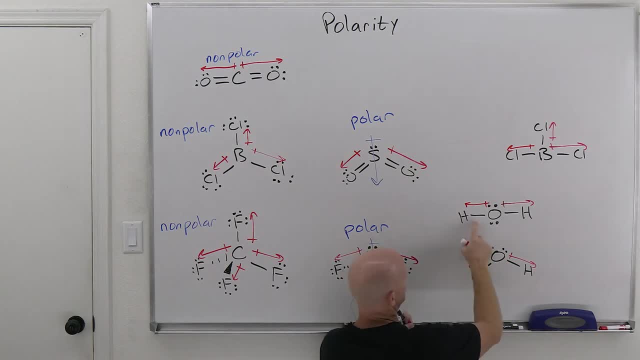 9.5 degrees apart. we learned, And, as a result, not according to what Mr Lewis shows, but what we know about the real molecular geometry. these don't cancel And, as a result, there's going to be an overall molecular dipole. 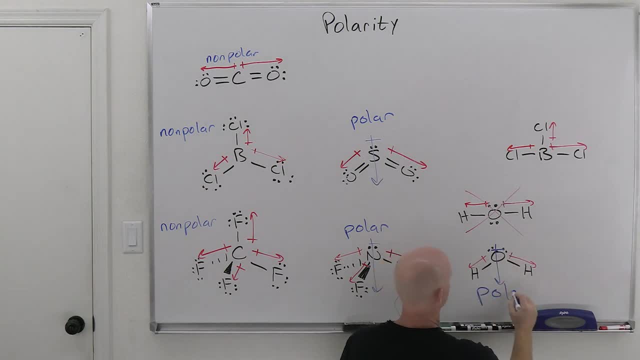 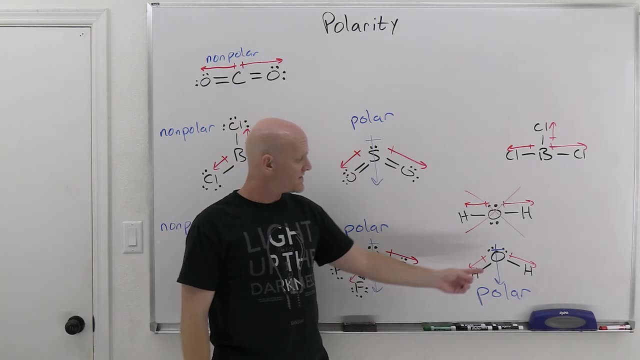 That's the average of those two, And this molecule is indeed polar. In fact, water is known to be really polar Cool. So yet another example where the central atom had lone pairs and it was polar, And most of the time. 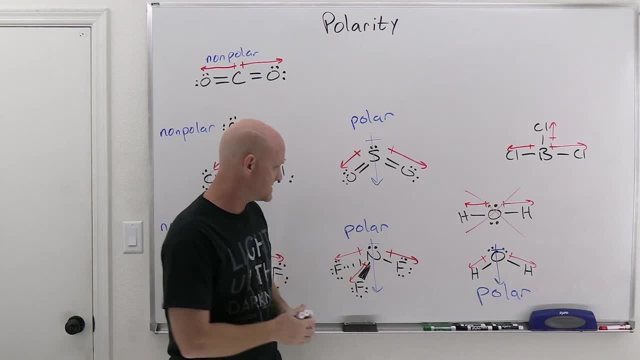 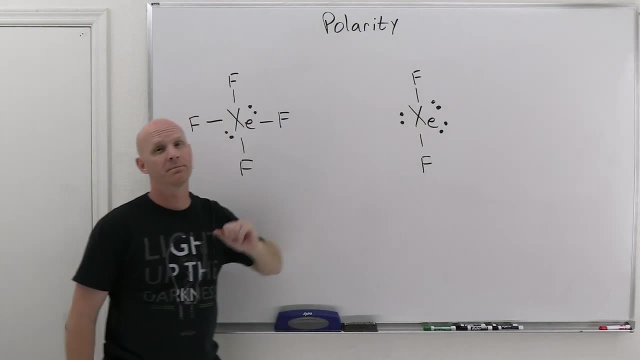 that's going to be the case, But I do want to show you a couple of exceptions. All right, Here's the two examples we're going to look at here. Notice: there are indeed lone pairs of electrons on the central atom in both cases. 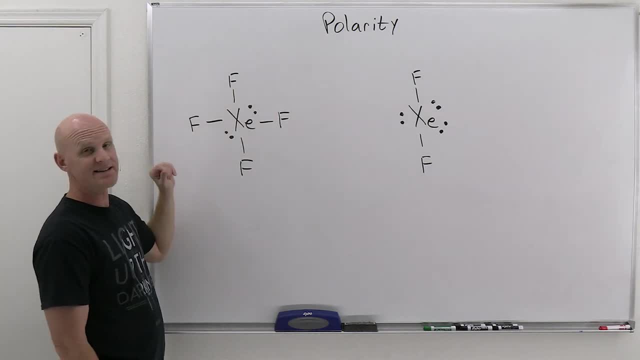 In this first one here. count up your total number of electron domains here And we've got six, four that are bonding and then two non-bonding domains, for a total of six. So the electron domain geometry is octahedral. 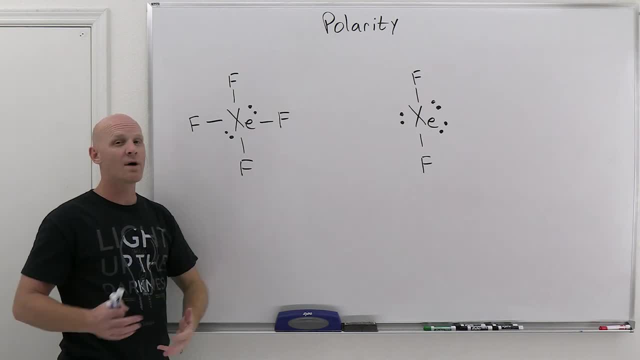 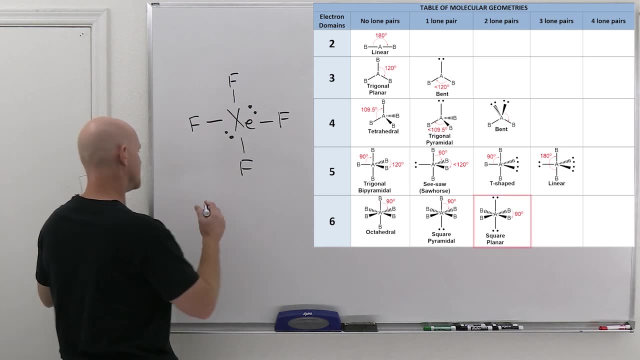 But the central atom having lone pairs, the molecular geometry will not go by that same name. And when you've got four bonding domains and two lone pairs, so that is going to be square planar. So with square planar you've got a certain degree of symmetry here. 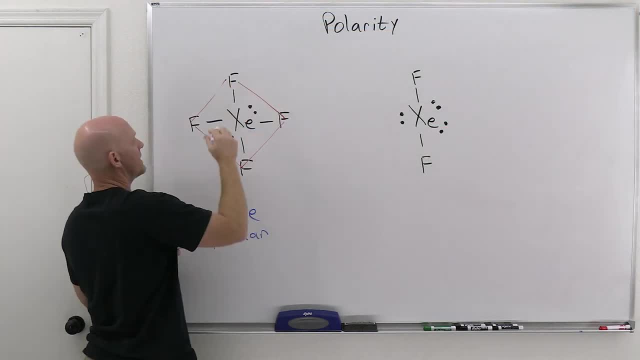 But these really do form a perfect square And so if you look at this polar bond, it's going to cancel perfectly with this polar bond because they really are 180 apart in this square planar structure. Same thing with this one and this one. 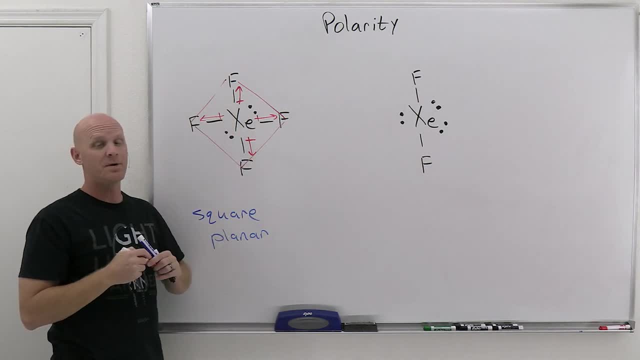 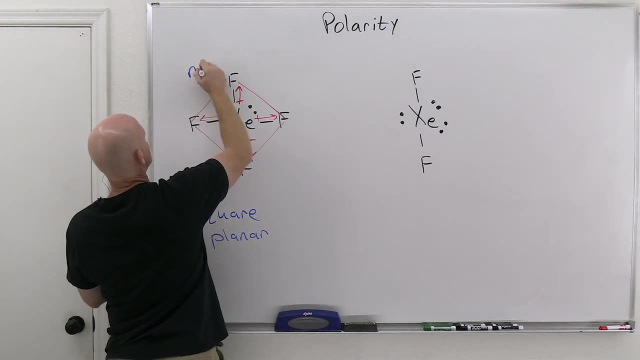 They're really 180 degrees apart when it's a square planar structure, and their bond dipoles are going to cancel, And so all four bond dipoles add up to zero, And so, as a result, this molecule is non-polar. 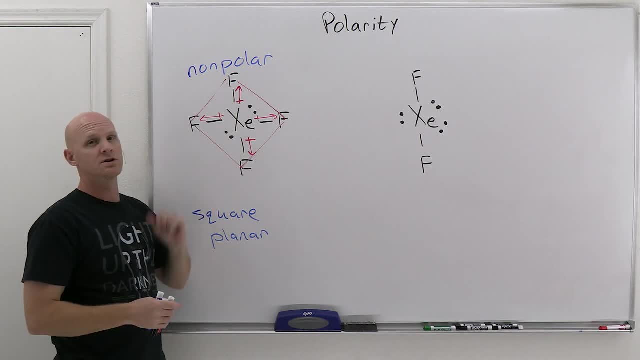 And a lot of students will get this wrong because they'll go Chad. it's got lone pairs And again, the rule is not that if you have lone pairs you're polar. The rule is, if you don't have lone pairs, 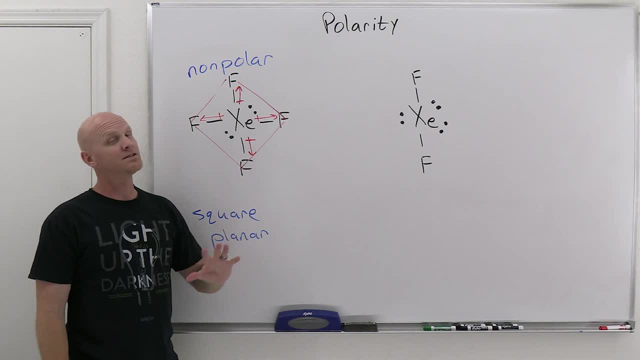 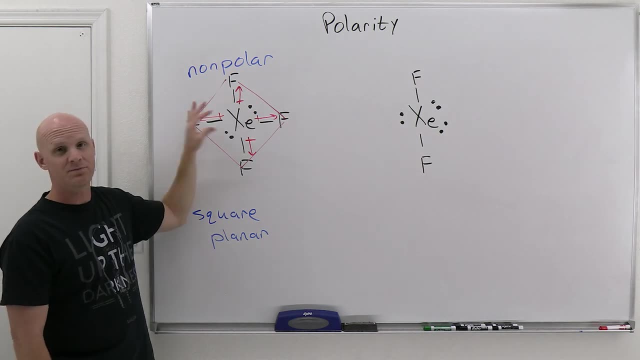 you're non-polar. But if you have lone pairs on the central atom it's probably polar. But here's your first exception. With the square planar molecular geometry it has a chance of being non-polar, assuming again, not just a chance. 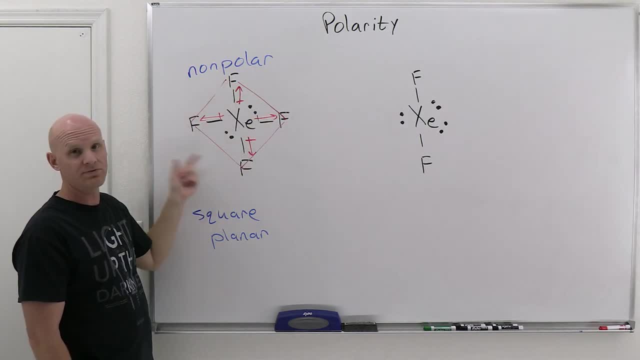 it will be non-polar if the outside atoms are all identical, In this case all fluorines in this example. Cool, we'll look at another one here. Here we've got five electron domains: two bonding, three non-bonding. 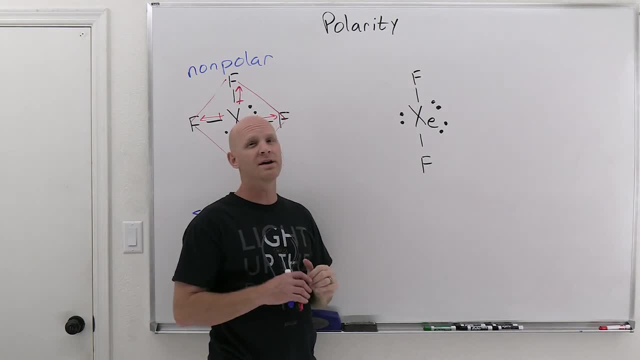 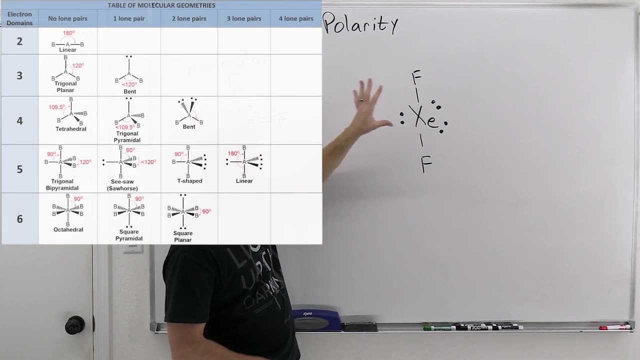 Five electron domains means trigonal, bipyramidal electron domain geometry And, once again, because the central atom has lone pairs, the molecular geometry goes by a different name And in this case with five total domains, two bonding, three non-bonding. 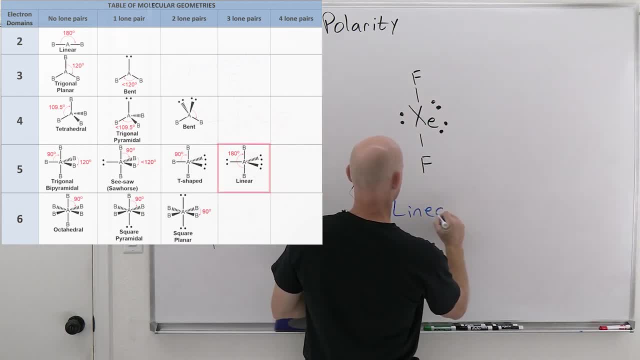 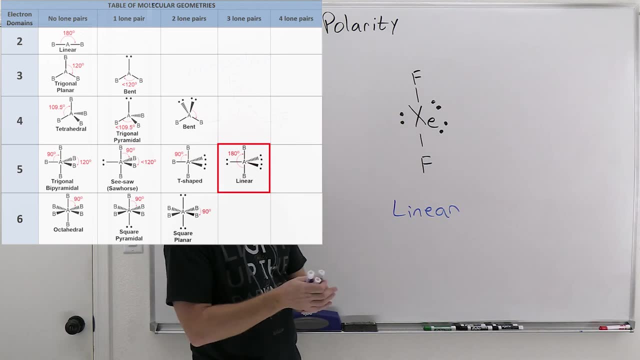 it is going to be a molecular geometry called linear, And that's important, because being linear in a straight line it means that these two xenon-fluorine bonds are 180 degrees apart, And so their bond dipoles are equal in magnitude. 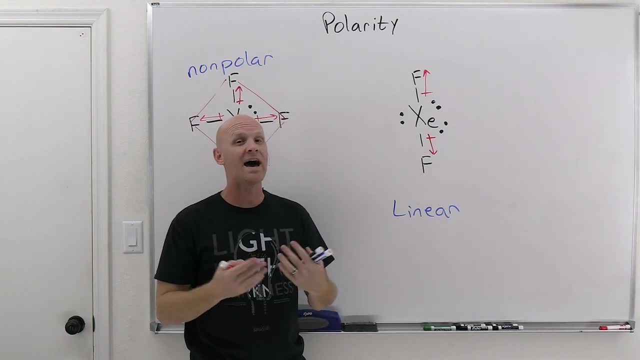 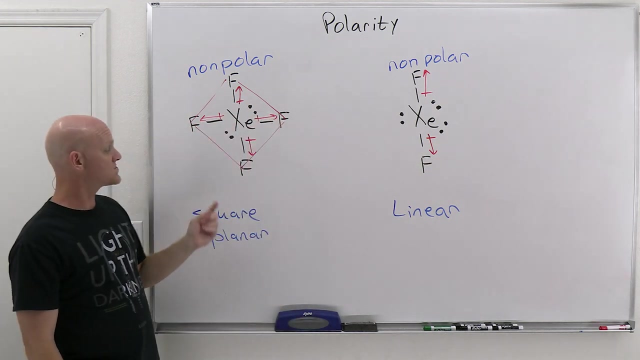 and exactly 180 degrees apart, opposite in direction, and add up to zero, meaning this is once again going to be non-polar, But it turns out this. is it So? the linear molecular geometry with five total electron domains or the square planar molecular geometry? 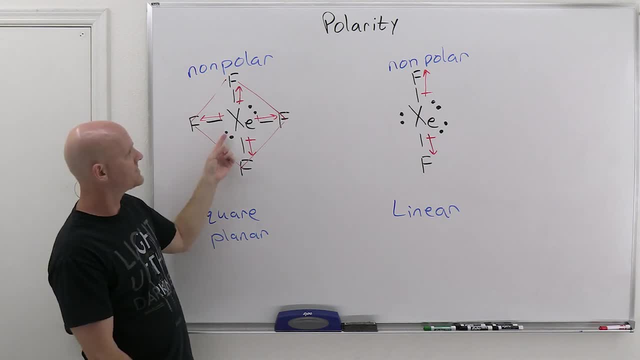 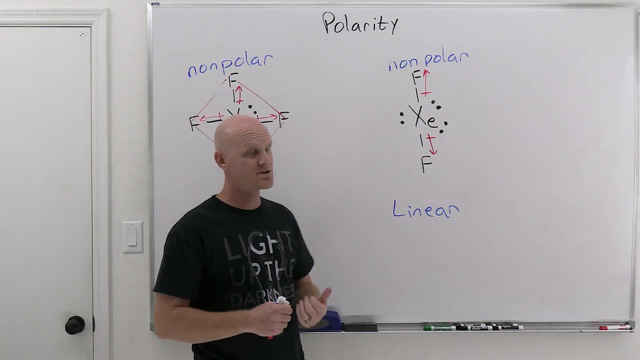 with six total domains. they are the two examples where you can have lone pairs on the central atom but still be non-polar. But all the rest of those geometries that have lone pairs on the central atom are typically going to end up polar. 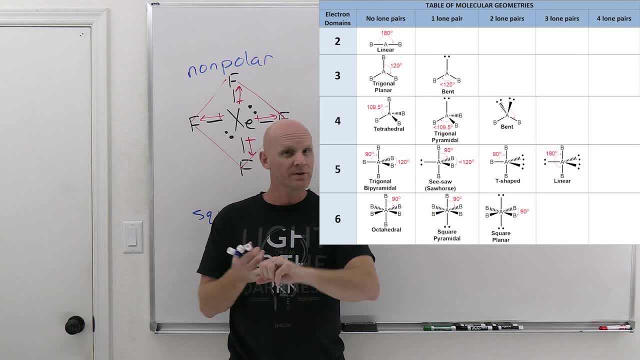 So like bent or trigonal, pyramidal or the other version of bent, with four electron domains, With five electron domains you could be looking at, like the seesaw or sawhorse That's typically going to be polar. What else we got there? 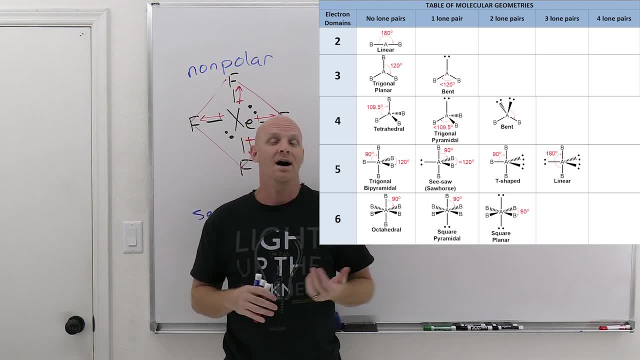 We got the T-shape- That's definitely going to be polar as well. And then, with six electron domains, you've got the square pyramidal, and that's typically going to be polar as well. All the bond tables don't cancel. 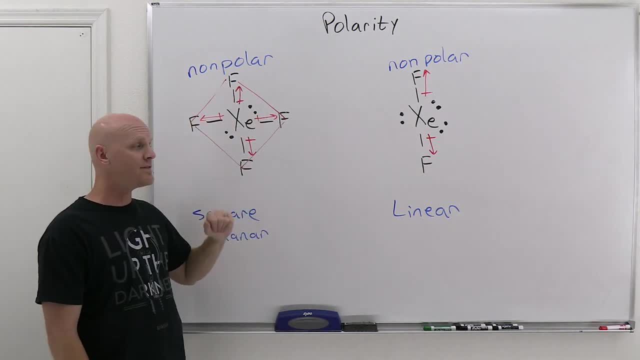 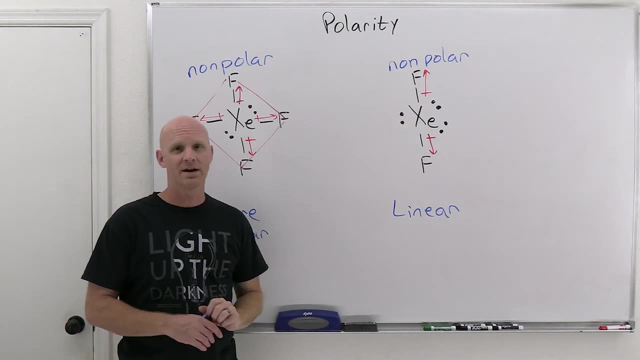 But again, the two examples with lone pairs on the central atom that still have a chance of being non-polar and typically are the square planar or the linear variant where it's got five total electron domains. So I just want to make sure you have seen that once before. 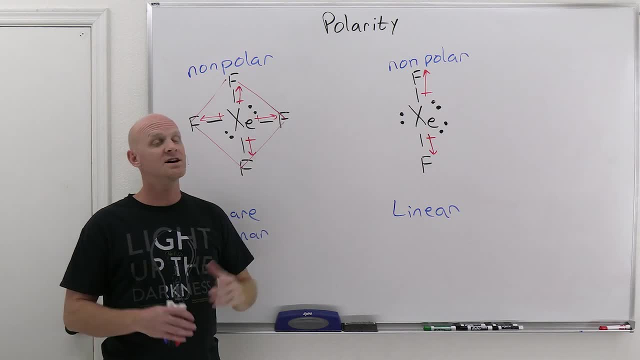 because, again, these two examples in particular are the ones that commonly show up in the test because professors expect you to have a better chance of getting them wrong. Now, if you found this lesson helpful, would you consider hitting that like button? It really helps to support the channel. 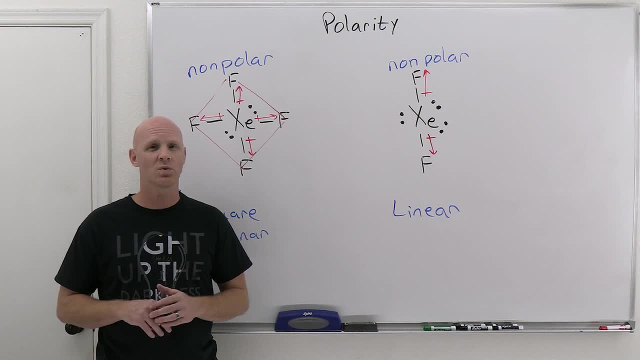 and lets YouTube know they should be sharing this lesson with other students as well. And if you'd rather not hit that like button, then my request of you is that you smile at a stranger in the next 24 hours, I know. spread that kindness. 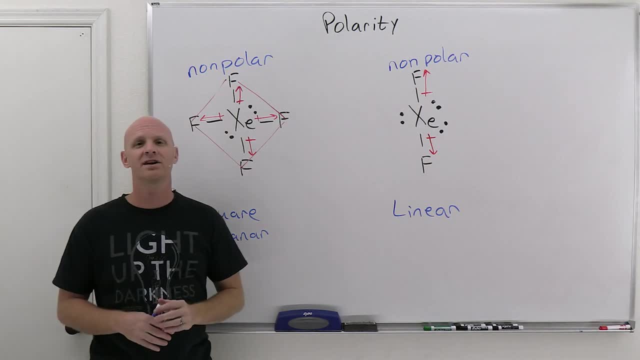 If you're looking for general chemistry practice, check out my general chemistry master course. Over 1,200 questions. so quizzes, chapter tests, practice, final exams. There are also final exam, rapid reviews and all the study guides come with it as well. 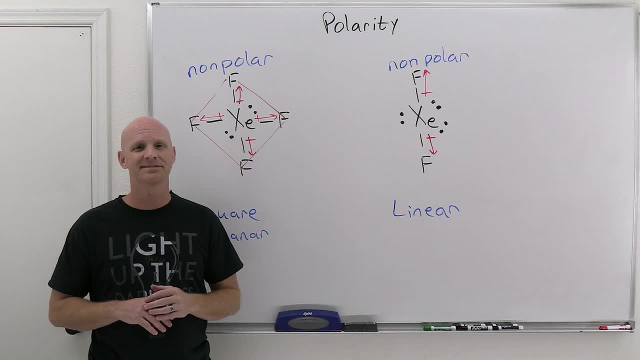 A free trial is available. I'll leave a link in the description. Thank you, Happy studying. 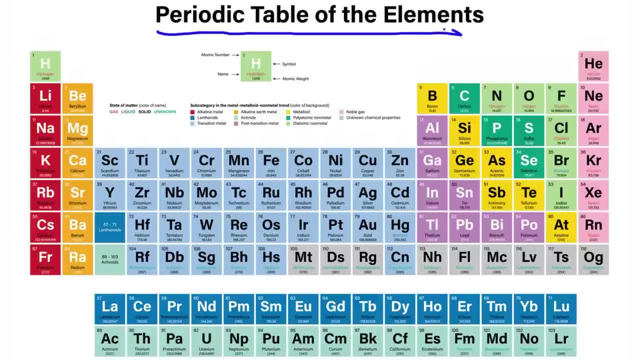 In this video, we're going to talk about the periodic table of the elements. Now there's two important things you need to know about this. The columns are called groups, the rows are called periods, So this is group 1, group 2,, 3,, 4,, 5, 6, 7,, 8,, 9,, 10,, 11,, 12, and so forth. 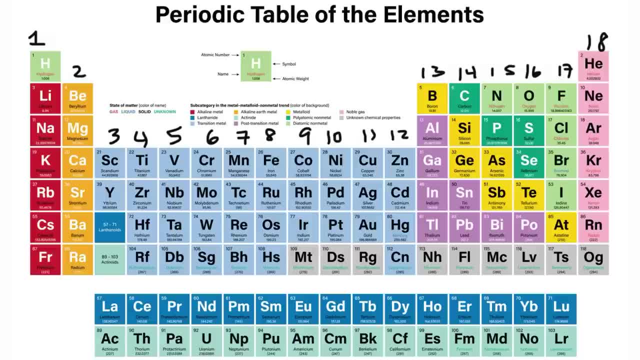 Now, the elements in a group share similar chemical properties. For instance, group 1 is known as the alkali metals. The alkali metals are the elements that are in the group 1,, 2,, 3,, 4,, 5,, 6,, 7,, 8,, 9,, 10,. 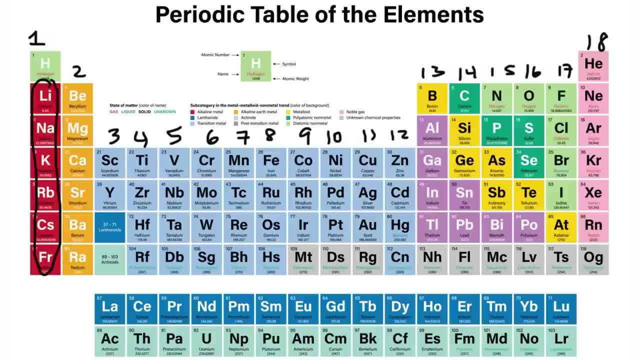 Include lithium, sodium, potassium, rubidium, cesium and francium. Hydrogen is not considered to be an alkali metal. The alkali metals, they're very reactive, All of these metals. they react violently with water. Some of them blow up with water. In fact, their reactivity increases as you. 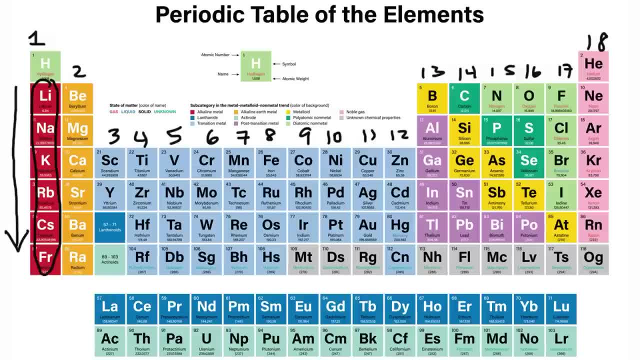 go down a group, which means that cesium is much more reactive than sodium. In fact, if you put cesium in water, it can blow up- There's a lot of YouTube videos that demonstrate this reaction- Whereas if you put sodium in.